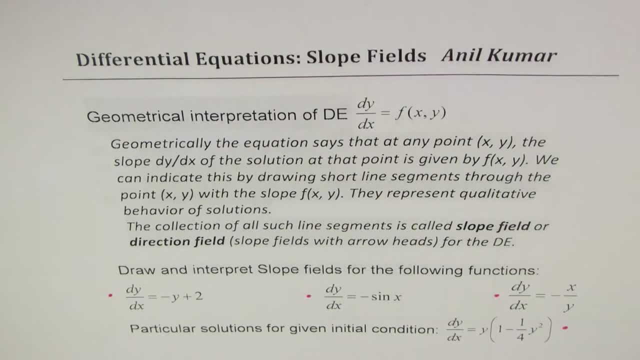 I am Anil Kumar. Before getting into details of solving differential equations, it is important to understand what they represent geometrically. So here we will talk about two terms. One is slow fields, the other one is direction field. They will be used. 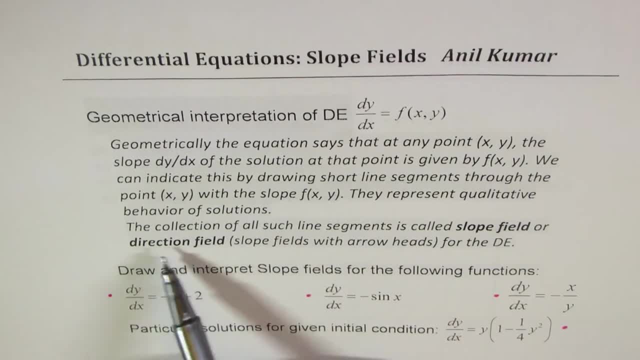 like in a very similar way. The only difference is direction fields, whenever you draw, will have arrowheads. The slow fields will be small line segments. Now, slow fields are graphical approach to look at all the solutions of a differential equation And slow fields consist of short line. 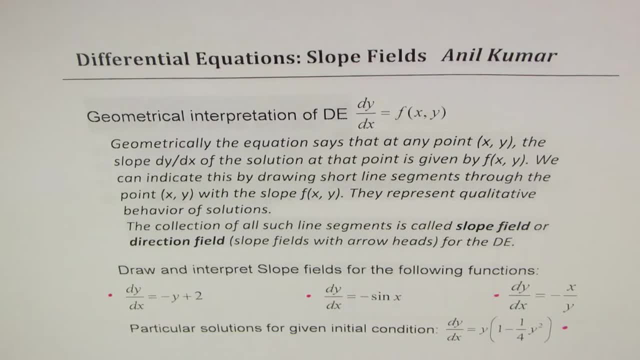 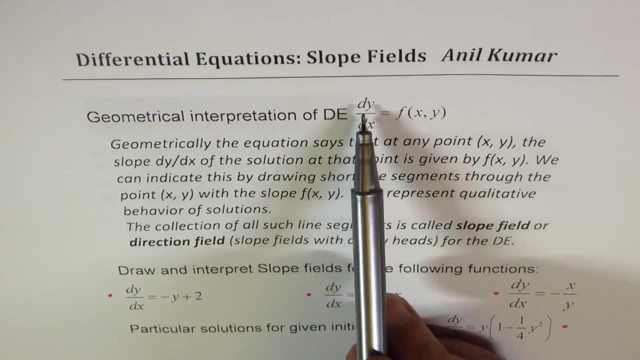 segments representing slope or steepness at the points x and y. So if you are given a differential equation dy dx equals to fxy, then you can geometrically interpret the as dy dx is a slope right. So at any point xy the slope at that point is given by the function. 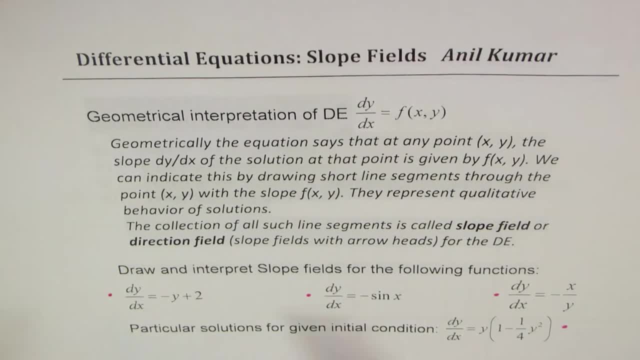 f of xy. So that is what it is. We will take these three examples and sketch slow fields for them and then interpret their meanings. The examples are: dy dx equals to minus y plus 2, dy dx equals to minus sin x and dy dx equals to minus xy. 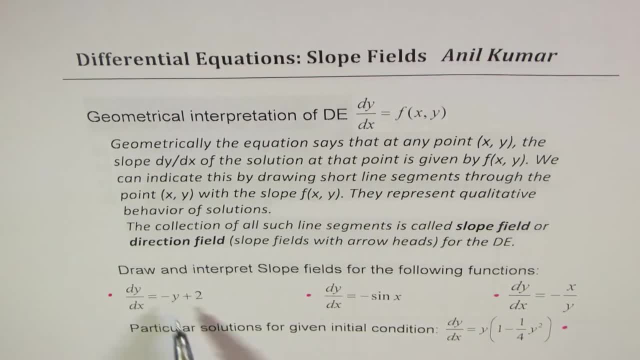 So here the slope is just a function of y, In this case it is function of x, And here it is function of both x and y. Then we will talk about in details slow fields and how to interpret a lot of. 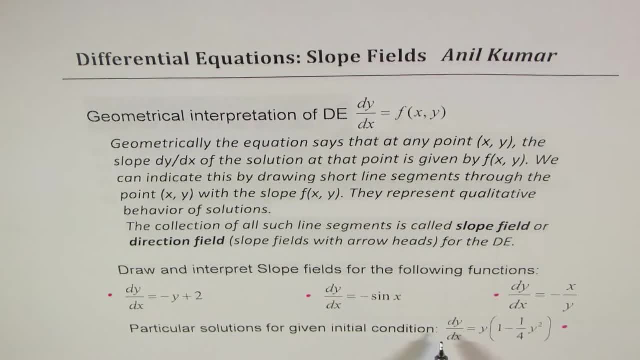 information a particular solution also when initial conditions are given. with the example dy dx equals to y times 1 minus 1 over 4 y squared. So let us take them one by one. The whole idea is only to understand slow fields and not really solve differential equations. 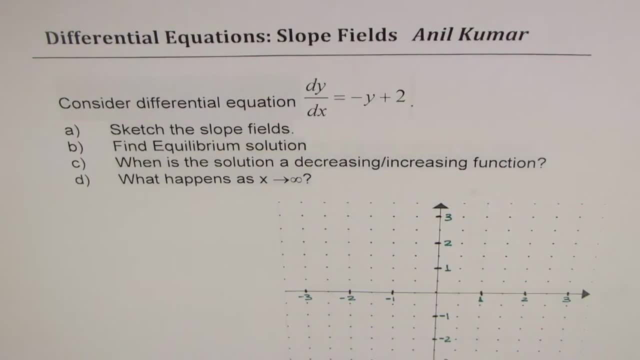 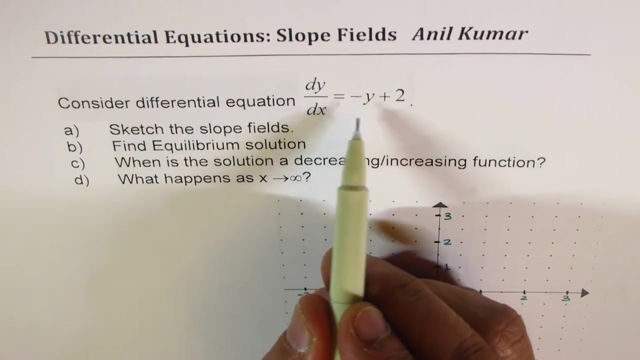 Here is the first example to draw slow fields. Let us consider the differential equation. dy dx equals to minus y plus 2.. As you can see the slope, dy dx is dependent only on y and is independent of x, correct? So here? 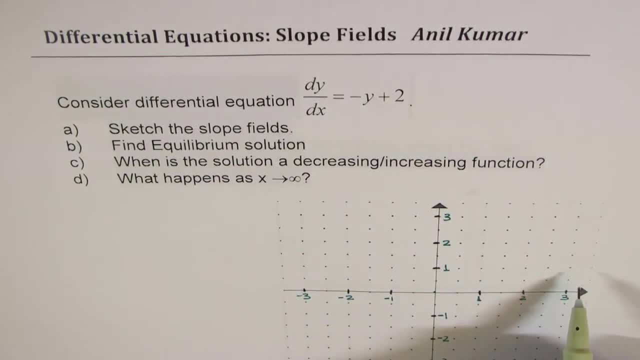 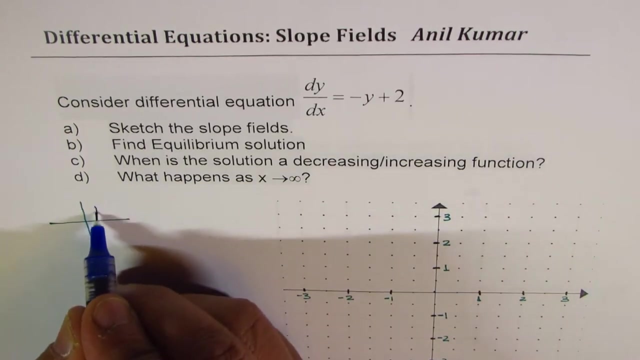 horizontally. if you move along, slope is going to be exactly same, correct. So whenever you have to draw slow fields, it is always a good idea to take the coordinate points. Now, since dy, dx, or rather I should say slope, is just minus y plus 2, independent of x. 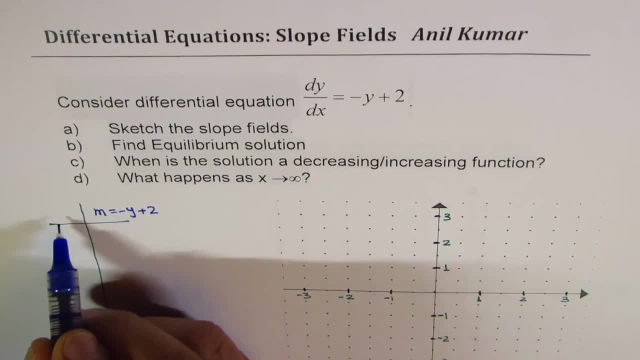 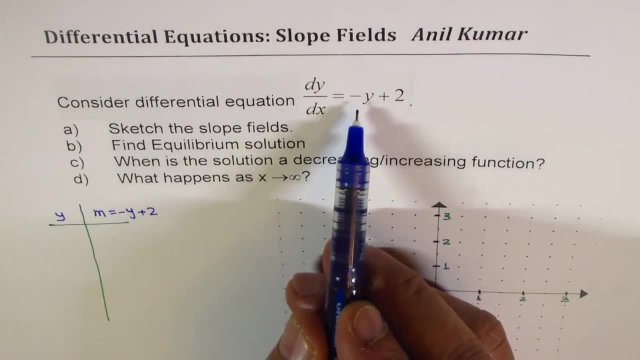 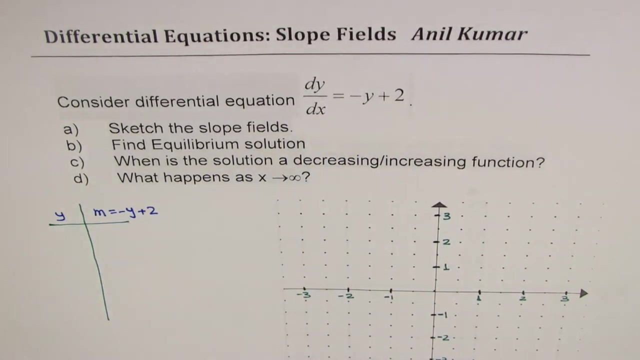 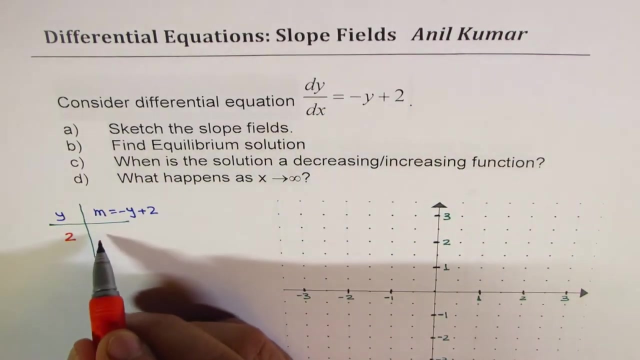 there is no point taking x values. So we will only consider the y values and we will calculate the slope. Always, to begin with we have to look for easy values. So first is y equals to 2.. So if I take a value of y as 2, for example, then minus 2 plus 2 is 0. Now 0 means horizontal. 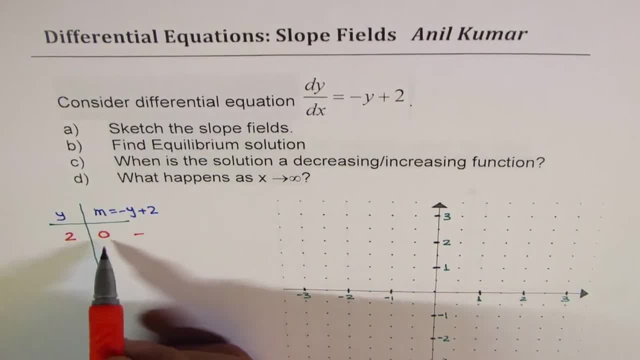 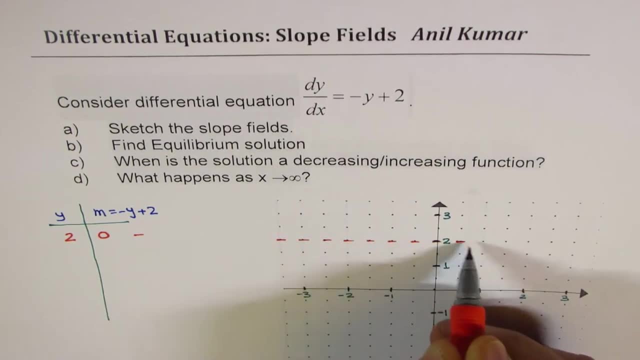 is going to be the slope right, That is 0 slope. So at y equals to 2, all these points we can mark horizontal short segments. These short segments are actually the slope fields for y equals to 2.. So any differential equation solution curve will be tange in to these points. That's the 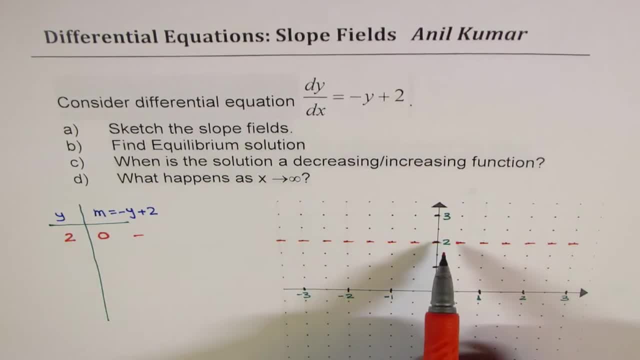 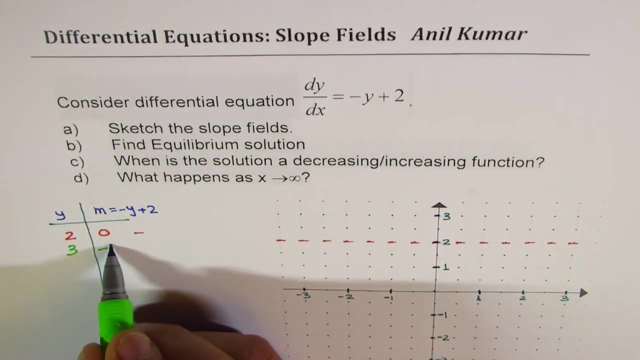 whole idea correct. Now, if I take a value more than two, let us say if I take a value which is 3, then what happens? If I take a value three minus 3 plus 1 is negative 1. so negative 1 means a slope will be going downwards, like this: 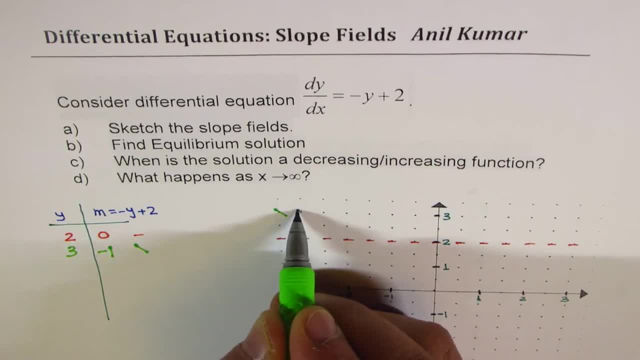 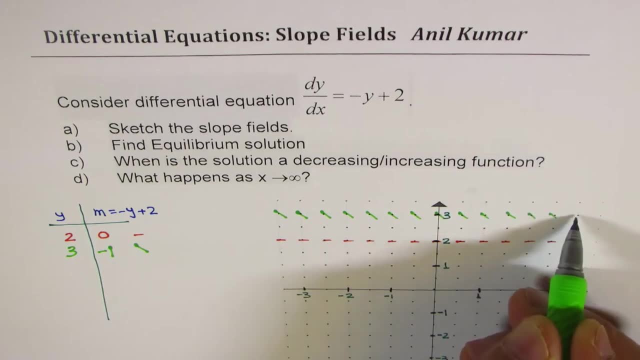 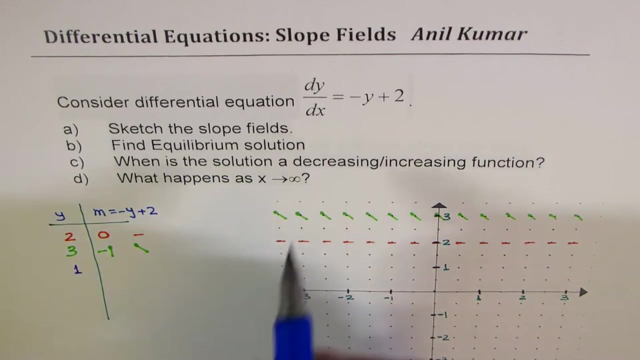 so all along this line we can draw short line segments with negative 1 slope right downward. you see that. so we get slope at all the points at where the y values 3. so if I take y value of 1 now for 1 minus 1 plus 2 is plus 1, so we get plus 1 means a slope. 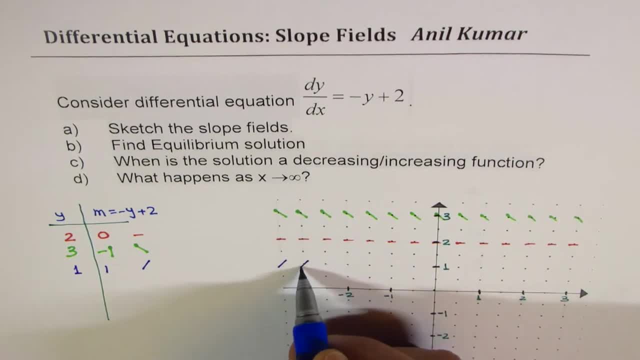 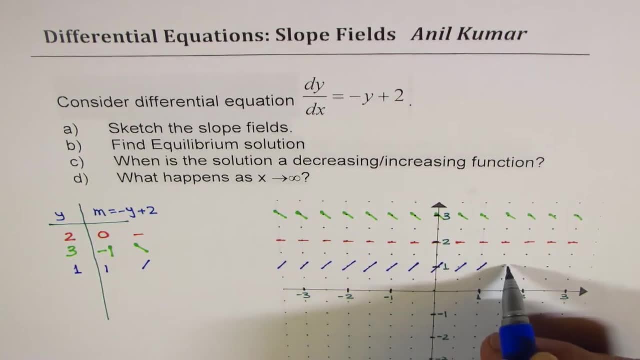 like this. so that means these short lines diagonal right. so this is: this is your slope 1. now, whenever we are drawing the slope fields, we don't put any arrows, but if we do direction fields, we put arrows. so that is another way of drawing the slope fields. so that is another way. 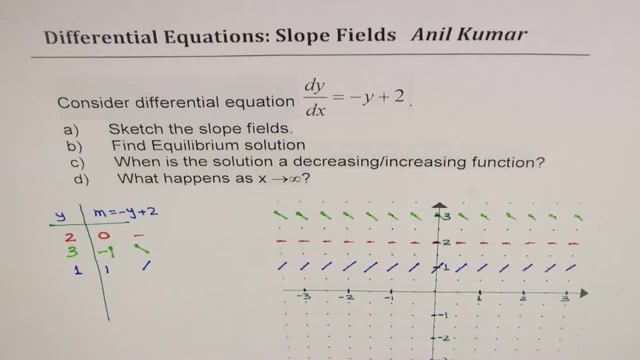 of drawing the slope fields. so that is another way of drawing the slope fields. so that is another way. the very subtle difference between the two. now, if y value is zero, then what? if y value is zero, the slope is two. two is steeper than one. so i'll make a line which is kind of like this: 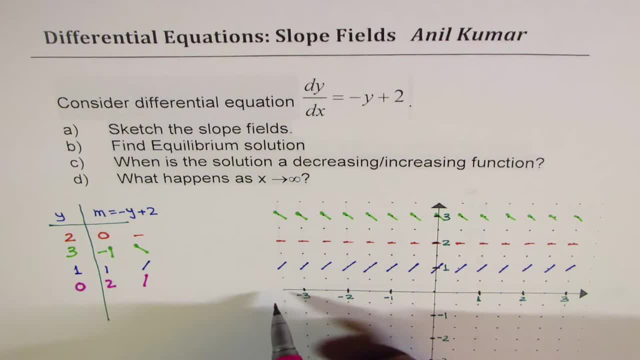 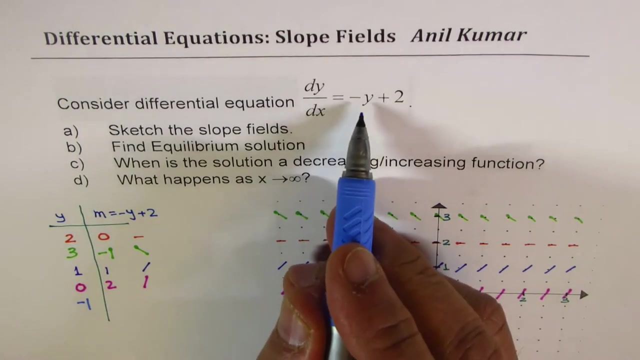 right? so all along the x-axis, the slope is going to be kind of like this, steeper than what we had drawn earlier. right, so that is that's how it is. so all along the x-axis, these are parallel short segments with slope of two. now, if i take minus one, then what minus one will make this? 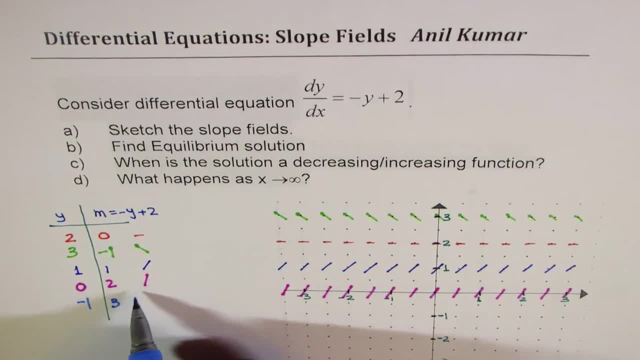 positive and we get plus three. so it is positive and three steeper than earlier. two right, so it is kind of like this. so at minus one it is even steeper than this. so let's go like this now. so what you observe here is that if the values are at two, we have horizontal slope. 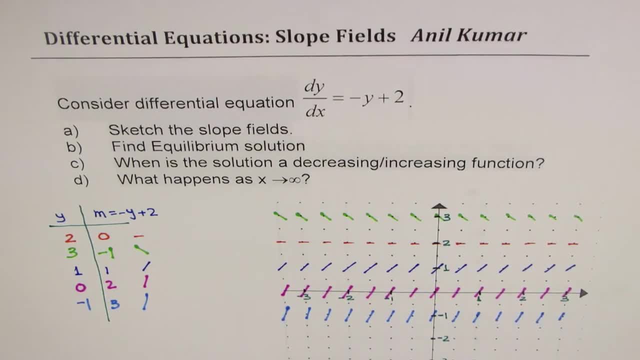 all the y values less than two positive slopes. and as we go down they are becoming steeper and steeper. do you understand? they are steeper and steeper. so if i take minus two, then minus two makes it plus two plus two plus four, and this is very steep. so we'll end here, actually. 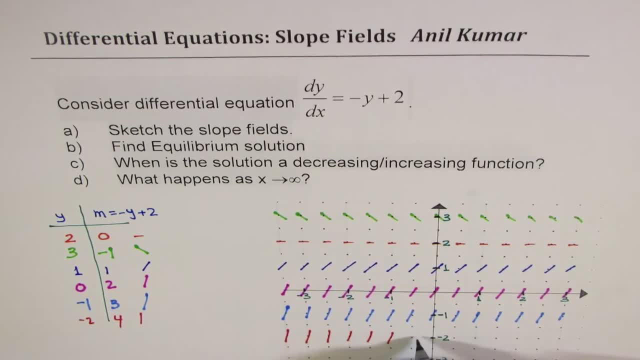 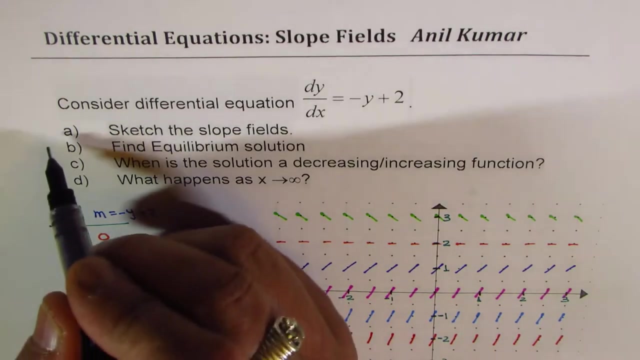 steep right, so that is what it is- almost like- a vertical line for me at present. right, so that becomes the slope. now i think from this pattern you can see a lot about the solution of your differential equation. dy, dx equals to minus y plus two. so we have done part one, which is 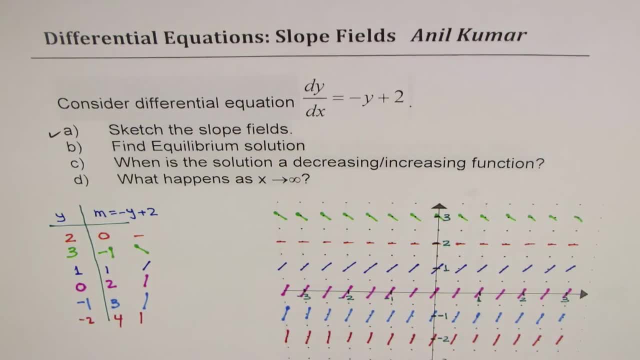 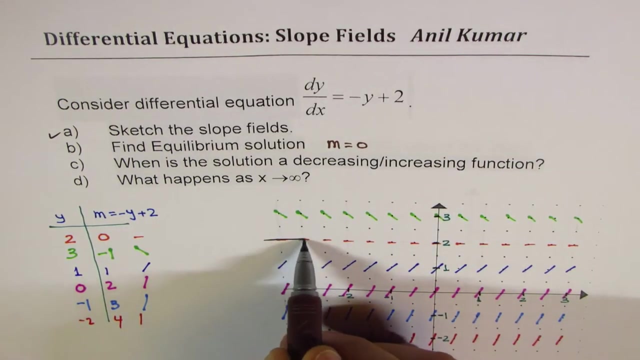 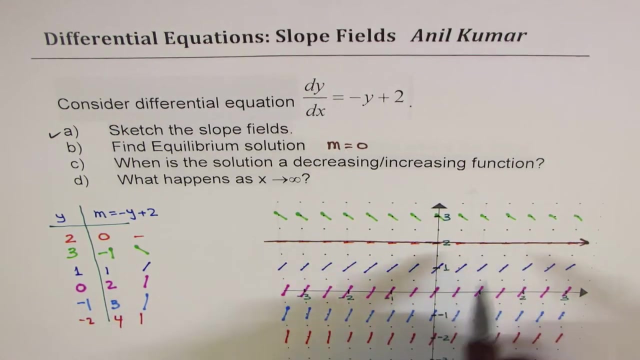 to sketch slope fields. now let's answer the next question: find equilibrium equation. what is that equilibrium equation? so when we say equilibrium equation it really means that the equation which is kind of horizontal, where the slope is zero. so from here the equation is this: that is equilibrium equation for the value y equals to two. 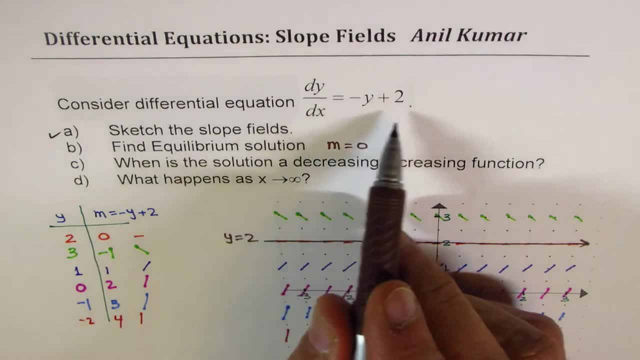 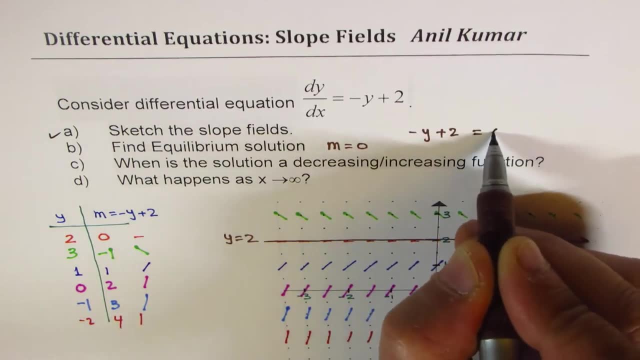 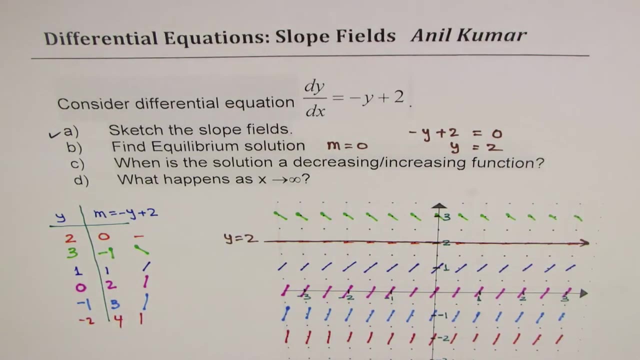 you will also get equilibrium equation by directly solving this equation. so what you could do here is you can equate minus y plus two equals to zero, and that gives you y equals to two as your equilibrium equation, right, so i hope that part is also absolutely clear. 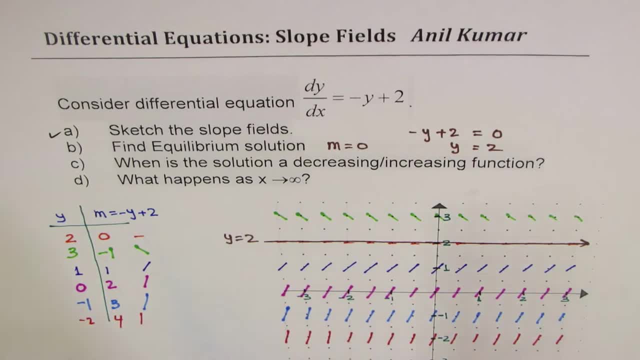 now let's look into the next question, which is: when is the solution? a decreasing or increasing function? so, as you can see here, if you have values more than two, the slopes are negative. so it is decreasing for. so let me write out clearly here: okay, so so decreasing for y greater than two, it is decreasing. 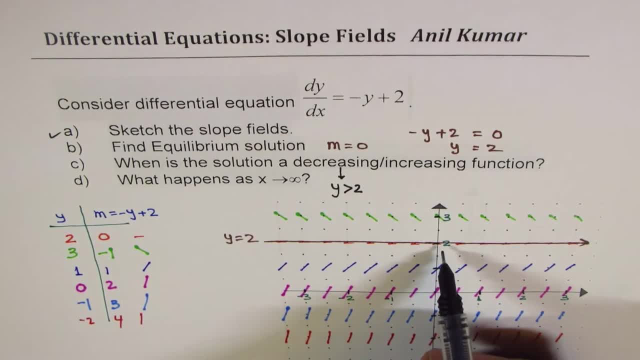 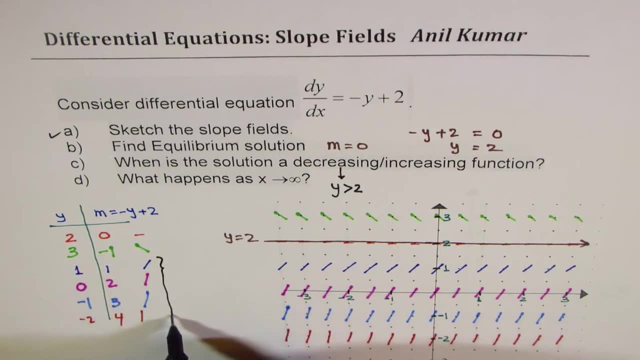 and when is it increasing? if the y value is less than two, all slopes are positive. correct, all slopes are positive. so all this: where y is less than two, we have increasing function, but if it is y is greater than two, in that case we have decreasing function. 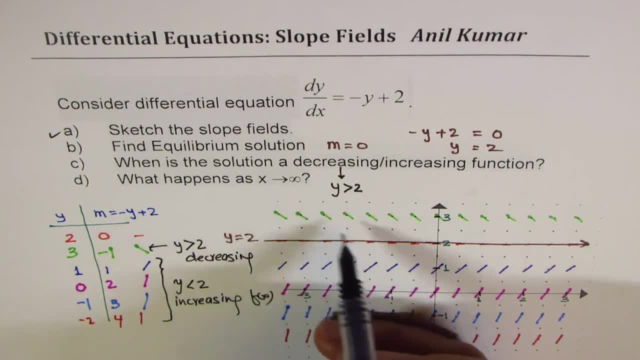 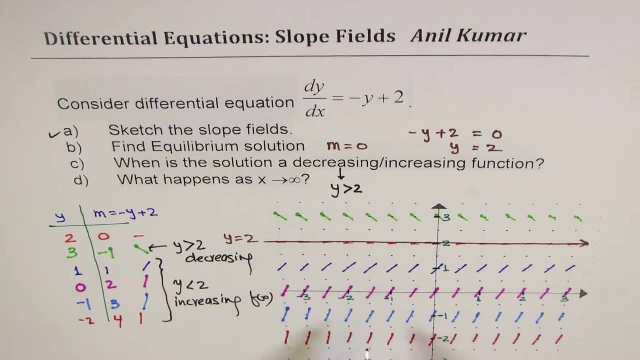 so i hope that is clear. decreasing because the slope is negative, so if i go to four it will be more decreasing, kind of correct. so that is how it is going to be. the last question here is what happens as x approaches infinity. now, if x approaches infinity, you see all these curves they actually approach towards. 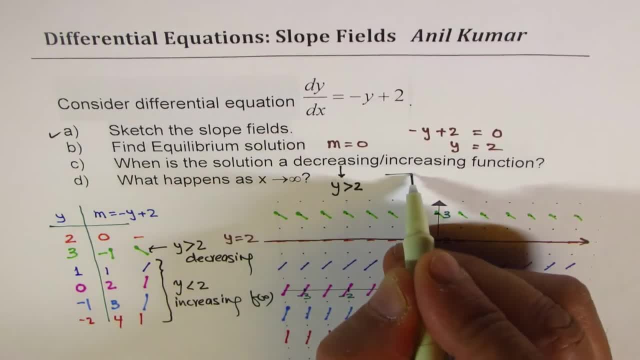 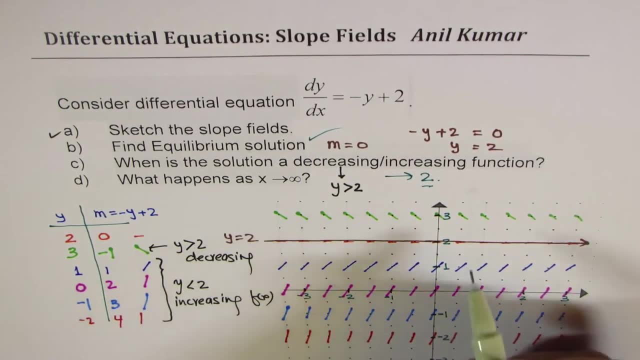 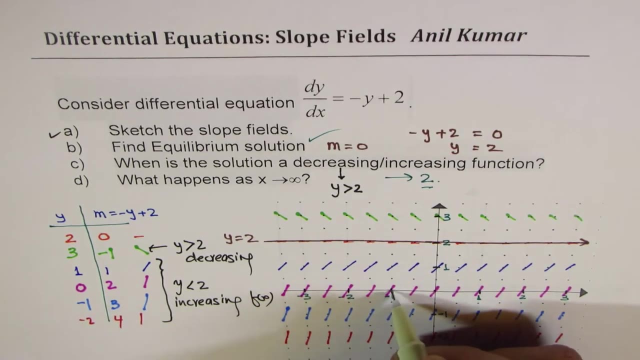 2, right? so when x approaches infinity, it approaches a value, 2, the equilibrium position. do you see that part correct? now you would always to draw a particular solution. what you could do is select a point. so if you select, let us say a point here which is at minus 1, 0. so if I select, 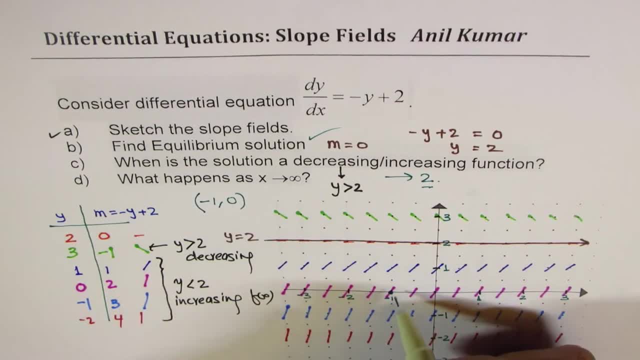 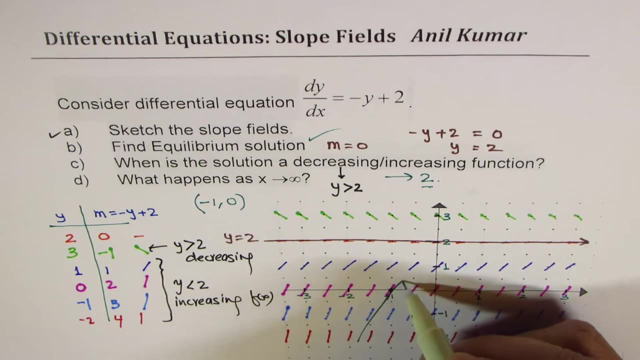 a point minus 1, 0, I could sketch a particular curve. the whole idea is, when you sketch a curve, then this segment should be tangent to your curve. so that is how you have to sketch it. so basically it will be kind of like this: so that curve indicates solution, a particular solution whose initial value is given to us. 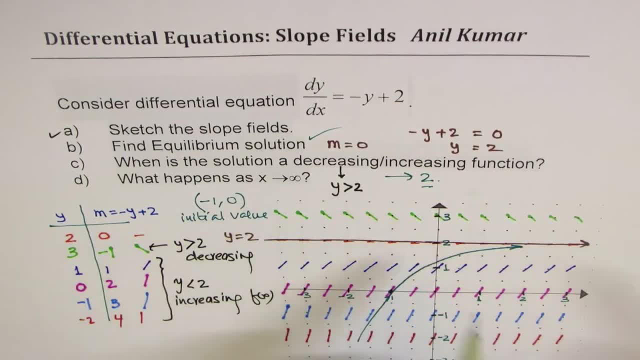 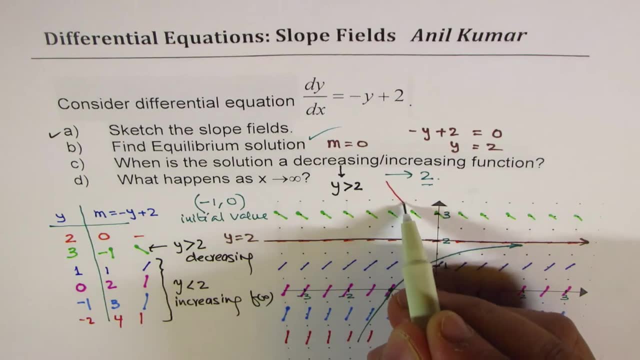 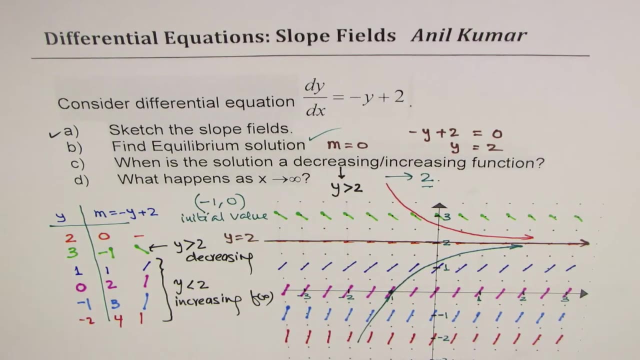 any of the curve you could select with some other value. for example, a curve above 2 will kind of look like this: decreasing, do you see that? so I hope that gives you a fairly good picture of what this is going to look like. so that is how you have to draw a particular solution. 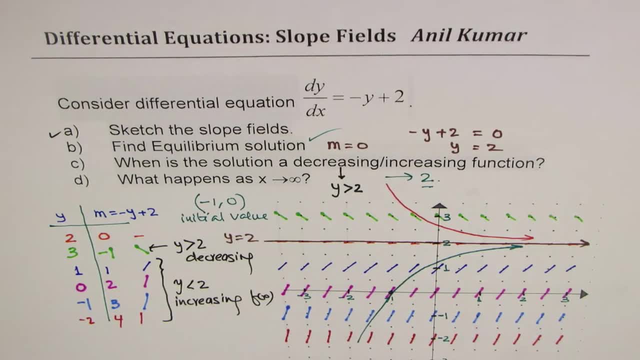 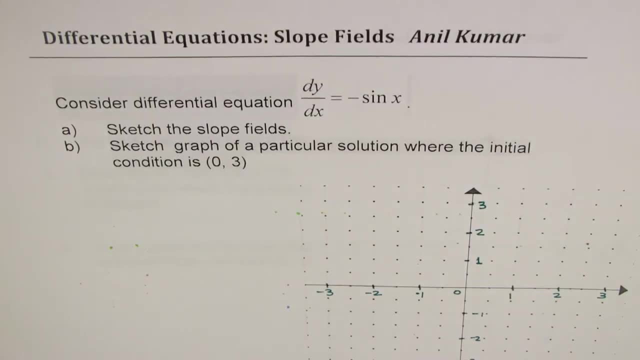 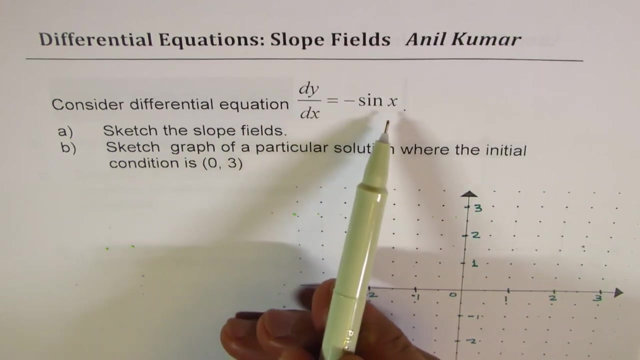 and this is the whole idea. now let us move on and take another example. this time we have a function where the slope changes with x. it is independent of y, correct? so let us discuss this now. now we will consider the equation dy: dx equals to minus sine x. we need to sketch the slope fields. 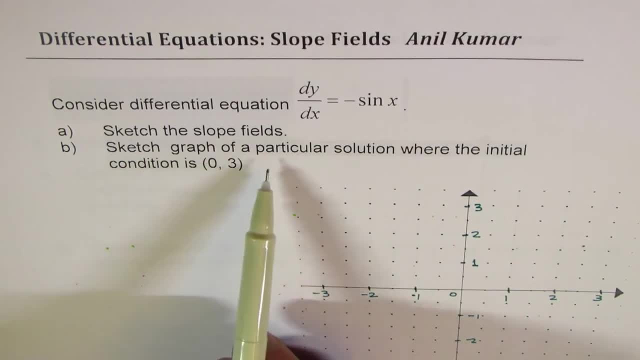 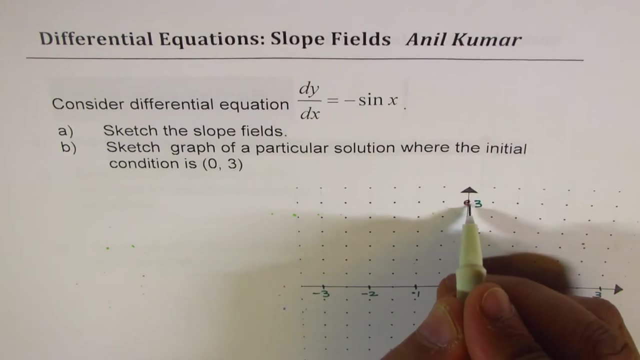 as we did earlier, and we will use the slope fields. as we did earlier and we will use the slope fields. need to sketch a graph of a particular solution where the initial condition is 0- 3. that means it will go through this point: 0, 3. right, that's what it has to be. we have to do so. first step is we. 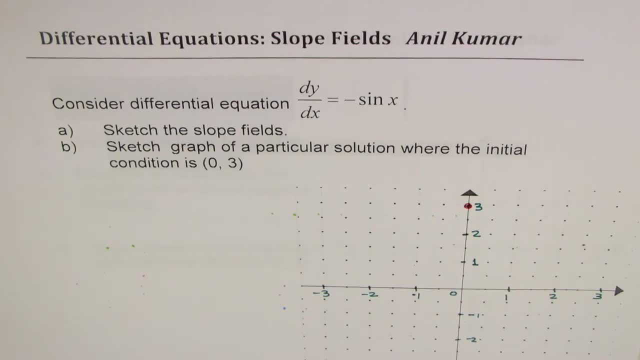 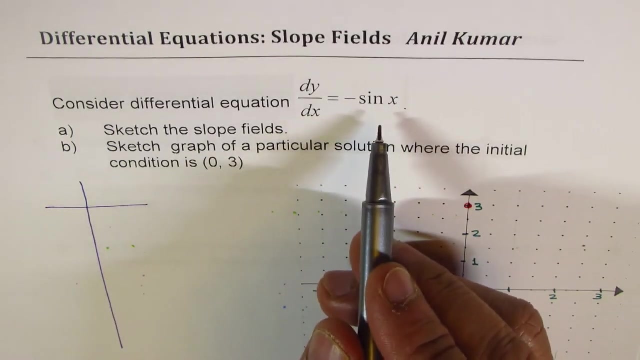 have to look at slopes at every point. so we'll consider a few points which are important to us, and from there we can draw the conclusion. let me first change the horizontal scale. when we talk about the trigonometric functions, we'll like to write the values in radians. that would be: 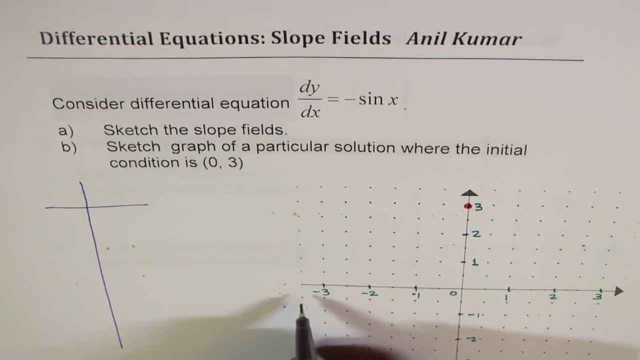 actually a better option, right. so, beginning from the left side to the right side, we could take values, let's say 0, in between, right, so we could go pi by 2 pi, 3, pi by 2, 2 pi. correct, so those could be values on the. 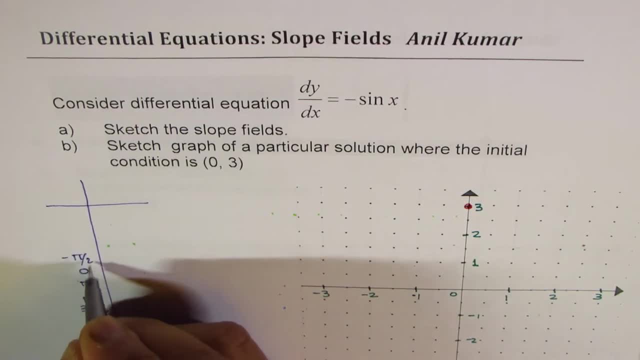 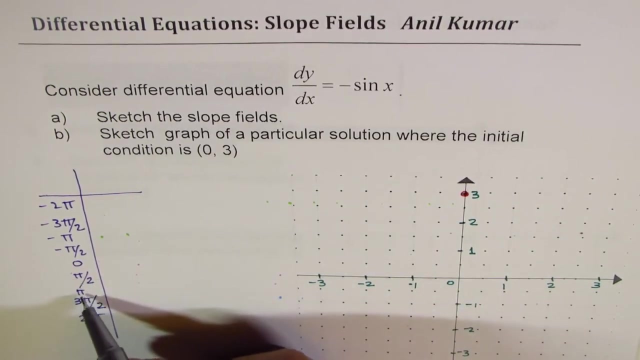 right side, and on the left side we'll go minus pi by 2, minus pi, minus 3 pi by 2 and minus 2 pi, is it okay? so those are the points which we are going to take, so i'll accordingly change. so we are having how many points? this is 0, 1, 2, 3, 4 on the right, so so i'll just change. 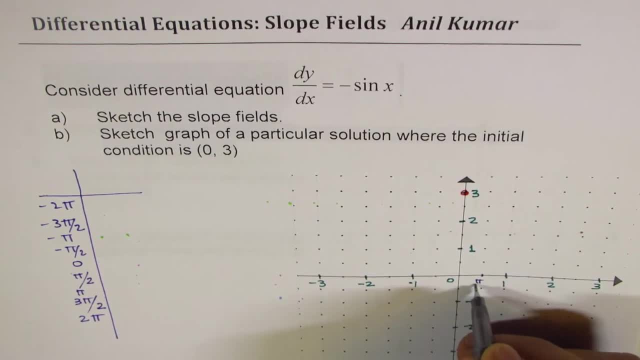 them right? so this we'll call pi by 2, then this will call it as pi, and then we have 3 pi by 2 and then W, and we write this as the root of 2. Pi over 2 and then W and we write this as 2 Pi. 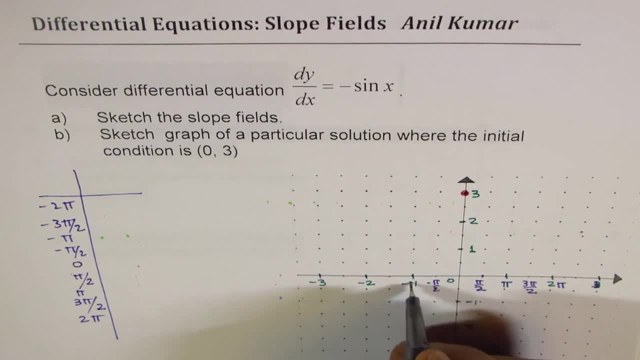 is it okay, forget about those. so we have this as: minus pi by 2, minus pi minus 1, pi by 2, minus 1 by 2 and 2 pi. so these are the values. so we have this as quite a short fourth time. okay, forget about those. 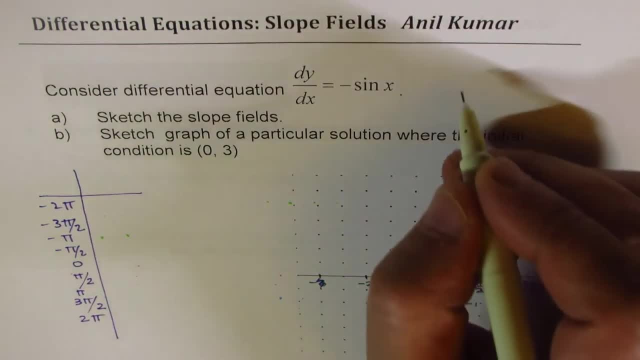 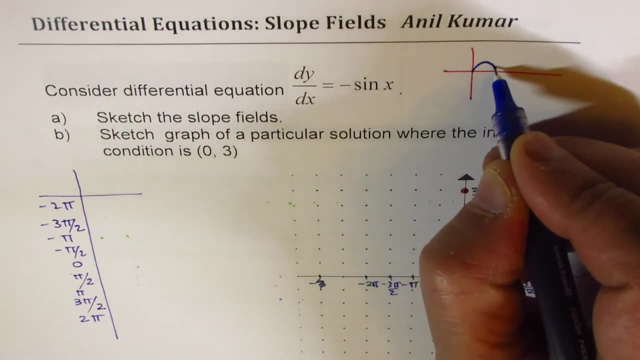 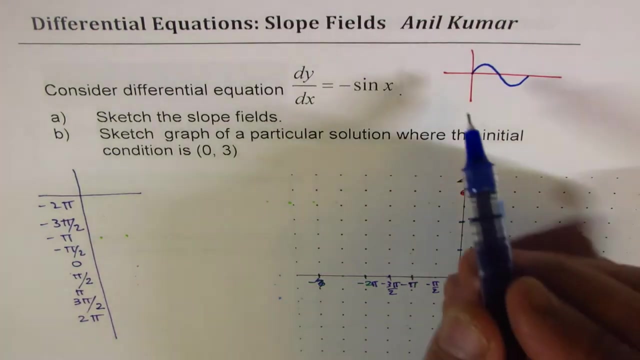 we look at the sine curve. let me just catch a sine curve on the side and that's easy to pick up. all the values. correct sine curve is kind of like this: remember, we have minus sine so I have to reflect it. but basically that is the sine curve right, 0 to 2 pi. okay, so let's take each and every. 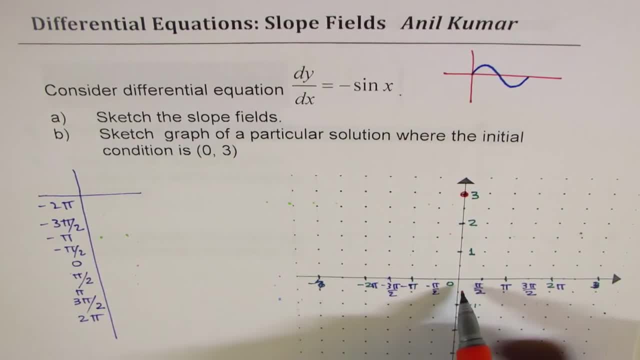 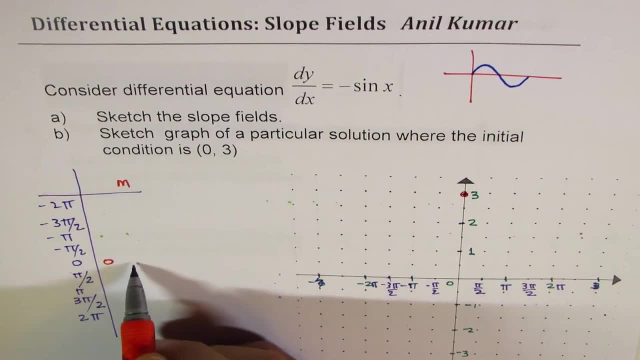 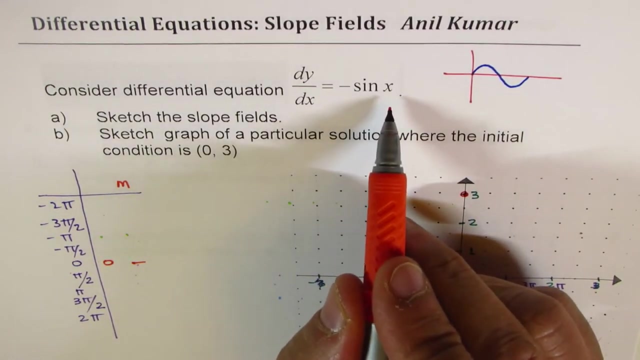 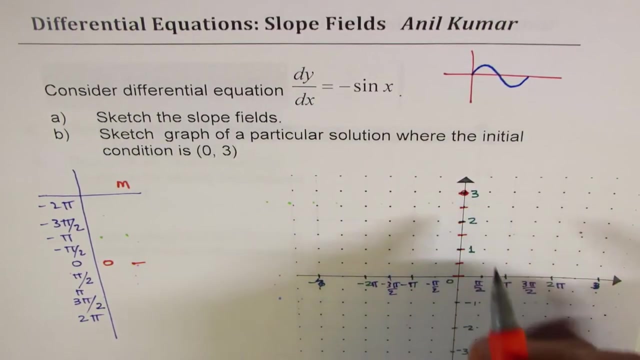 point starting with with 0. so sine of 0 is 0, so sine of 0 is is 0. that means we are talking about slope, which is horizontal. so wherever it is 0, it is going to be horizontal, since y values are not changing the slope. so as we go higher up, it is going to remain horizontal. or as we go down below. 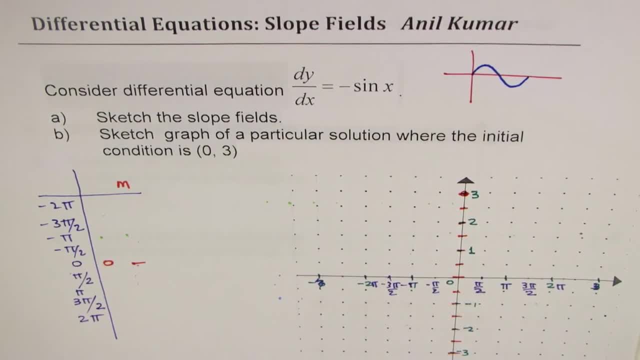 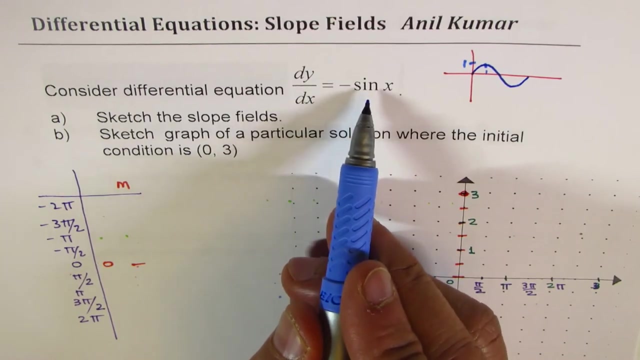 it is going to remain horizontal, right? does that make sense? okay, so that's one. now let's take another point, which is pi by 2. so at pi by 2, the y value is 1 minus 1, since we are working with minus sine x. so here it is going to be minus 1. that means 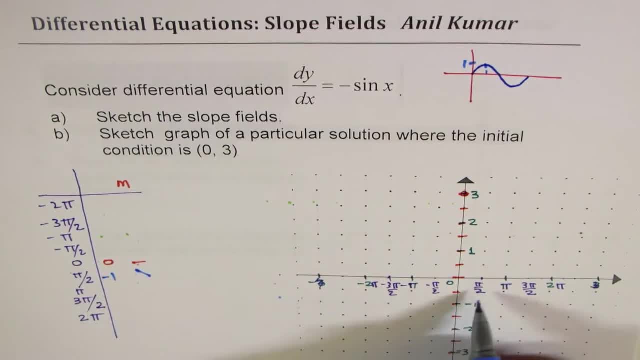 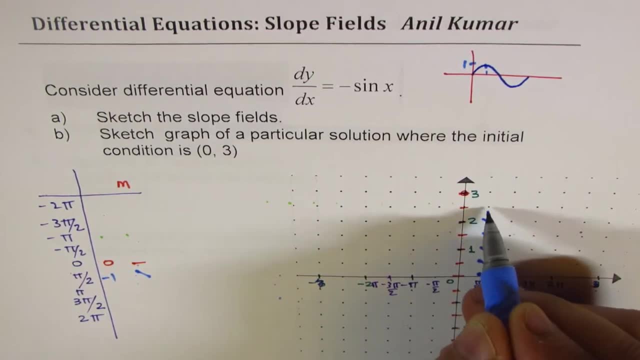 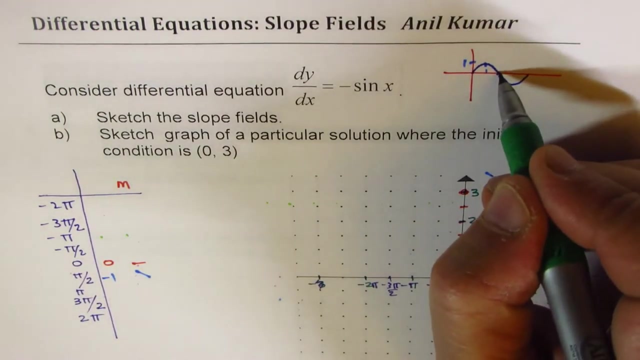 downwards like this, so at pi by 2, the it is a downward slope. like this, so all along, x equals to pi by 2. the vertical will have that kind of slope dropping down correct. now let's take the next value, which is pi. now, for pi sine is 0, so pi sine. 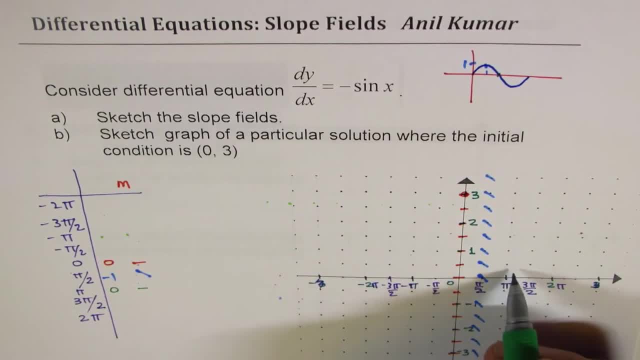 is 0, it again means horizontal. so we again have horizontal at pi. so all these values will be horizontal. then 3 pi by 2. now when we talk about 3 pi by 2, we are looking at a value which is minus 1 right. 3 pi by 2 is: 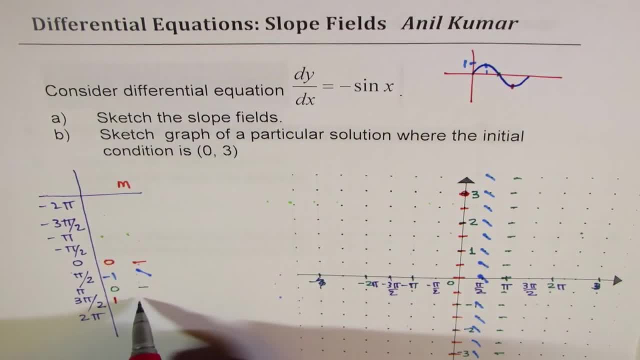 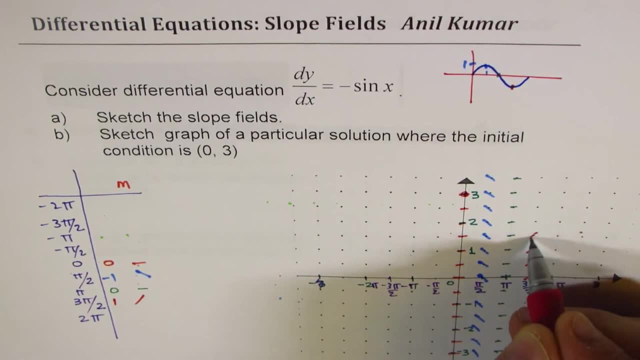 minus 1. but minus of minus 1 gives us plus 1. that means upwards. so 3 pi by 2 it will be short segments will be kind of like this: correct, and at 2 pi it is again 0.. 0, 0 means horizontal, right. so we'll discuss, we'll just draw horizontal line segments for 2 pi. 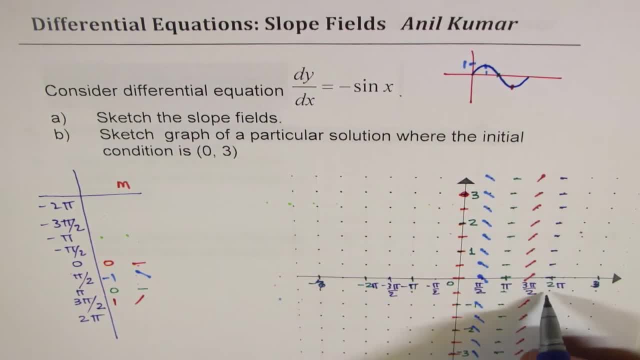 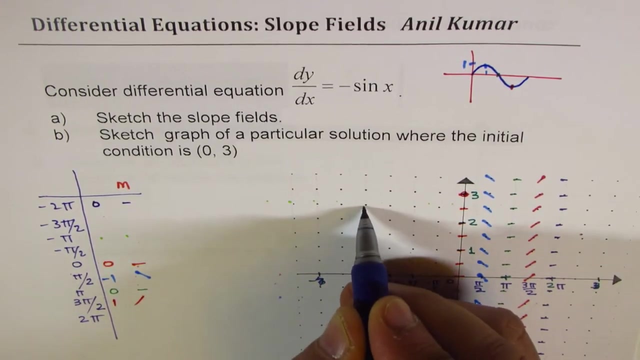 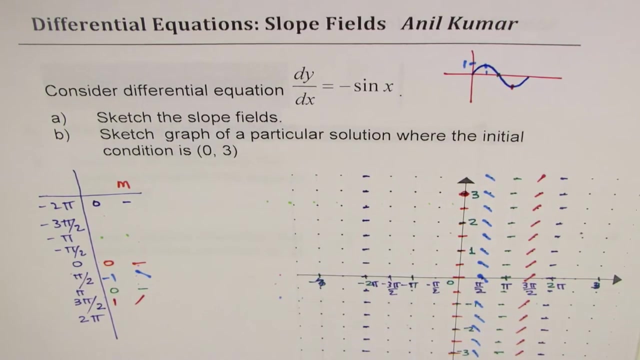 correct. so let's start from the other side. minus 2 pi is also 0. that means horizontal. minus 2 pi is right there. so we get these horizontal lines all along the line. vertical line x equals to minus 2 pi, correct, as far as minus 3 pi by 2 is concerned. well, this graph actually. 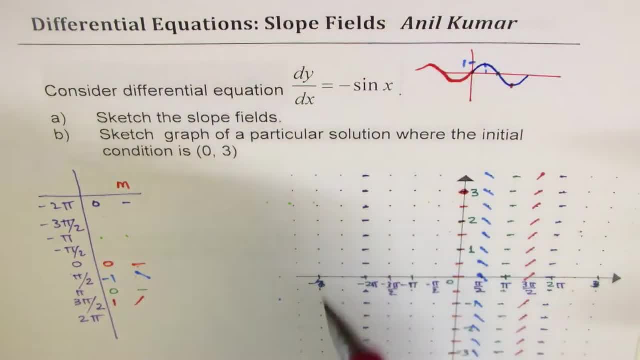 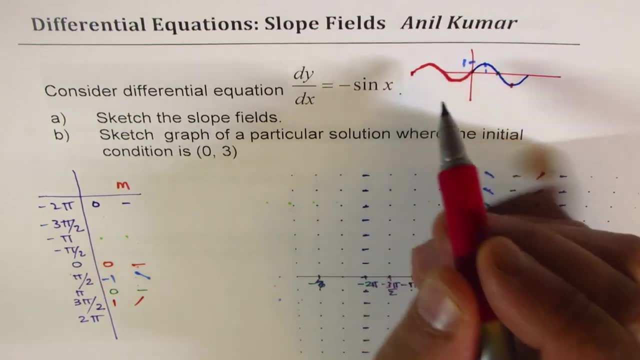 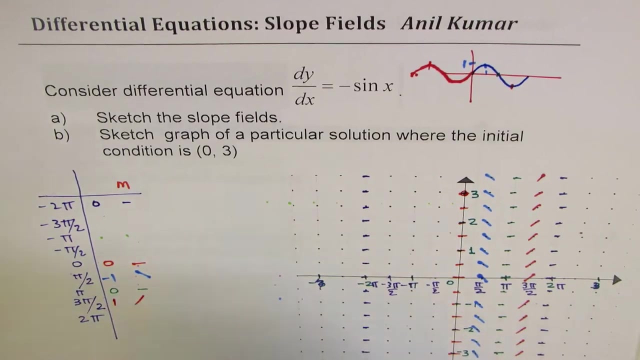 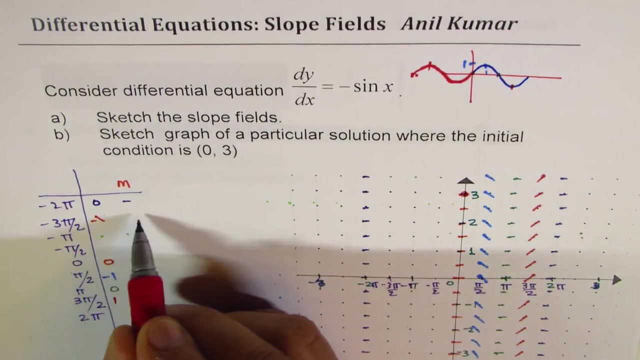 repeats like this, right, so symmetrical. now. minus 3 pi by 2 means this is: this is like come here. so this is 2 pi, correct. and minus 3 pi by 2 is positive 1. so that means minus positive 1. but negative means negative here, right, so negative 1 means it will be dropping. 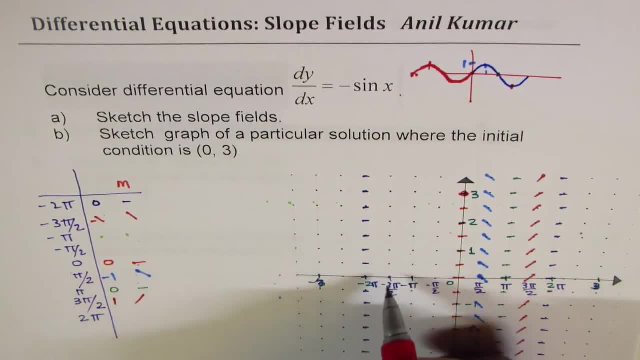 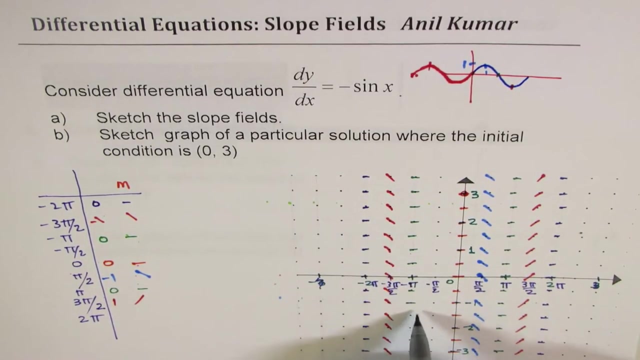 down like this. so we have a slope at minus 3 pi by 2, which would be like this: then, at pi minus pi again, it will be 0. so at minus pi it is 0 horizontal line and at minus pi by 2 it is negative 1, which will give us negative and. 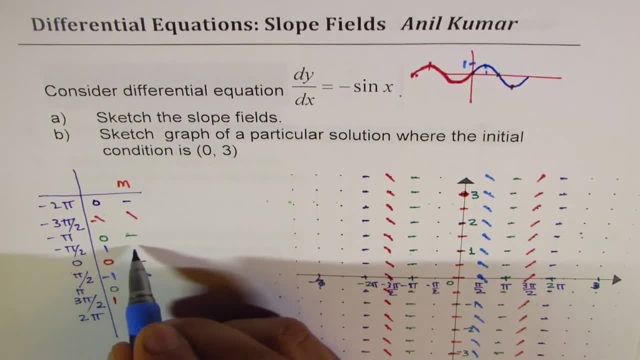 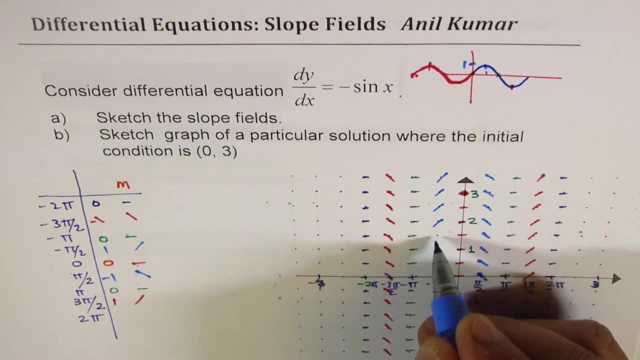 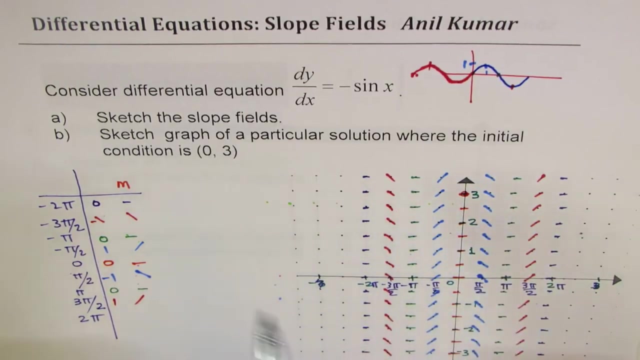 negative becomes positive 1, so that would be positive 1 and that means like this: So positive slope of 1, a diagonal short segment gives you the slope field at minus pi by 2.. So that is how we get our field, as you can see here. right, that is how it is. 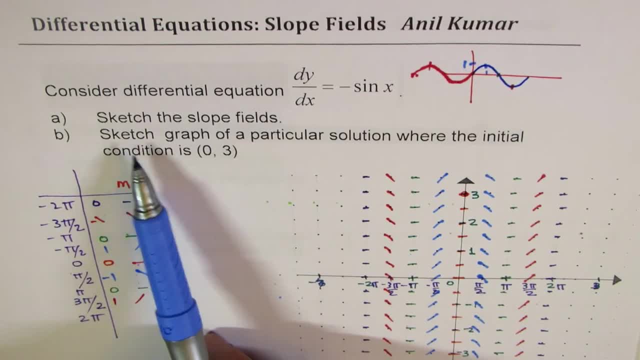 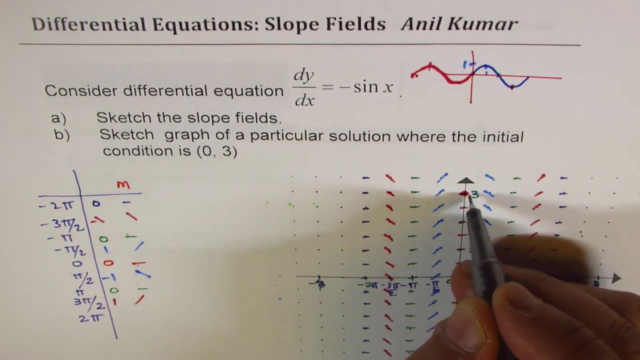 So we have sketched the slope field. part b is sketch graph of a particular solution where the initial condition is 0, 3.. Now here we have 0, 3 as our initial condition. Now if I have to sketch a graph, it is horizontal here on the left side is coming down on the 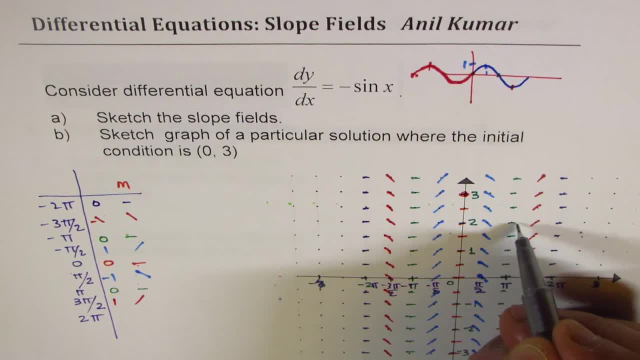 right side also, it is coming down and then it has to turn from here. so those horizontal are the turning points correct. So how do we sketch it? So let us do that. So what we will do here is that we will sketch. this becomes a tangent to our curve and it 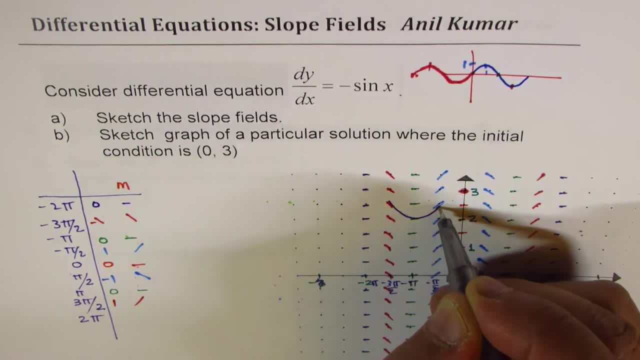 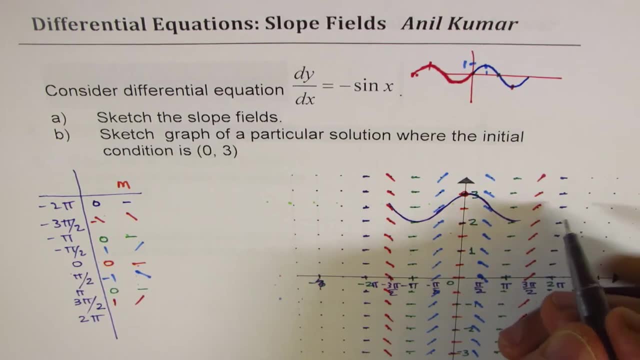 has to turn like this. so it is kind of like this. do you see that? So that is how it is going to be. so it will turn from all the horizontal points and these short segments are the tangents. so you have to be very careful in all these short segments. 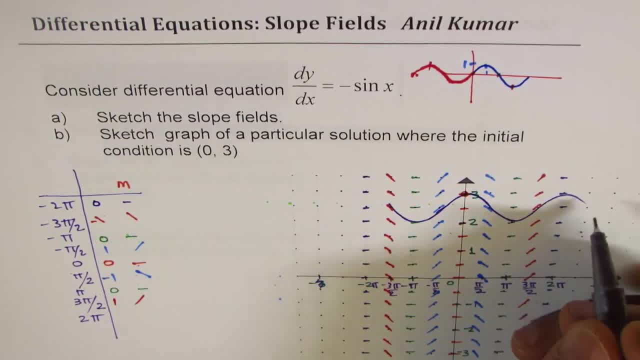 will become the tangents as you go along. Now, since you start with the maximum, it is a cosine function, correct? So that is the solution. you know, derivative of a cosine function is minus sine x, so it makes sense. So that is how we can look at the solution from the slope fields. 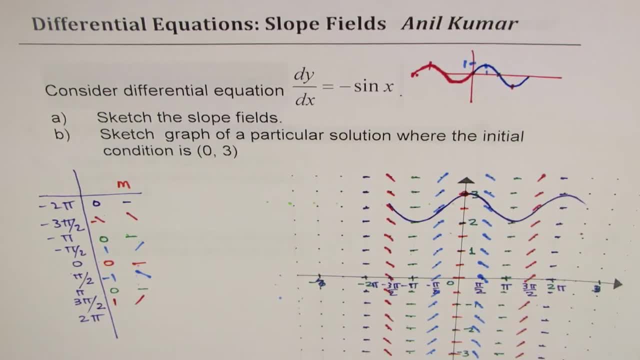 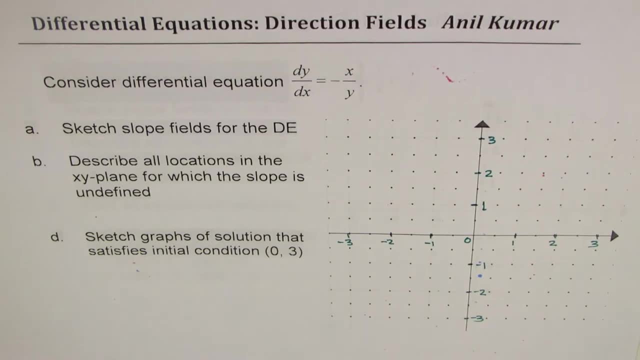 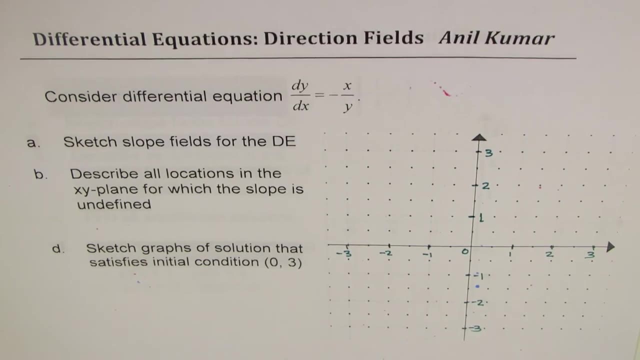 So I hope this point is well taken care. Now let us take the next example, and then we will do a question in more details. So as we are moving along, we are adding some complexity. We began with function Which was independent of x, then we took the trigonometric function, which was independent. 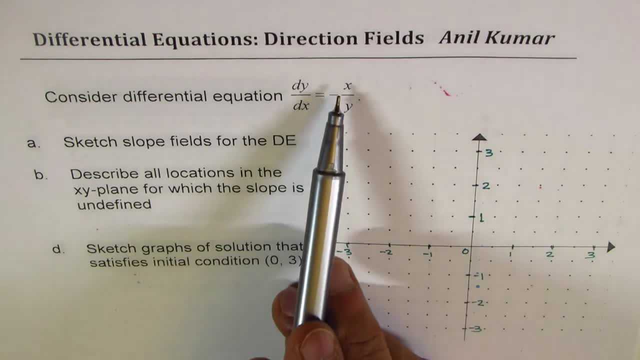 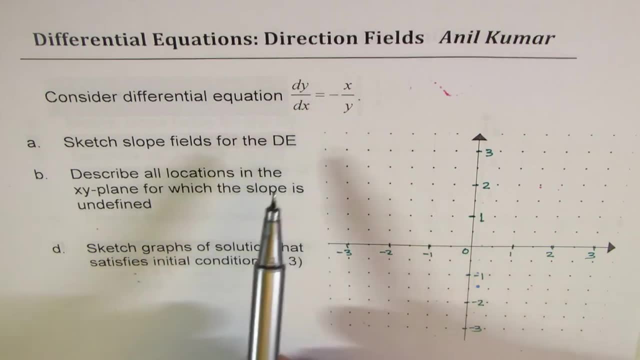 of y, and now we have a function which depends on both x and y. So we will consider the differential equation. dy: dx equals to minus x over y. Now here we need to sketch the fields for the differential equation, describe all locations in the xy plane for which the slope is undefined, and then remove one part. 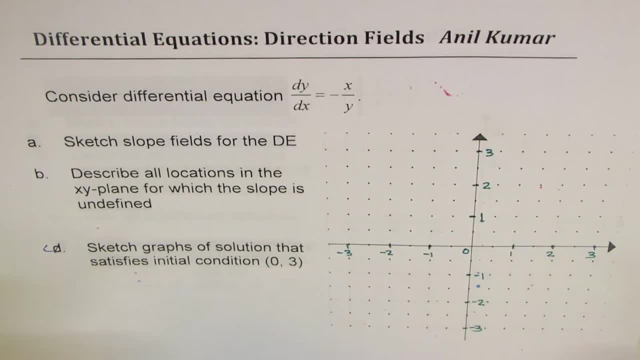 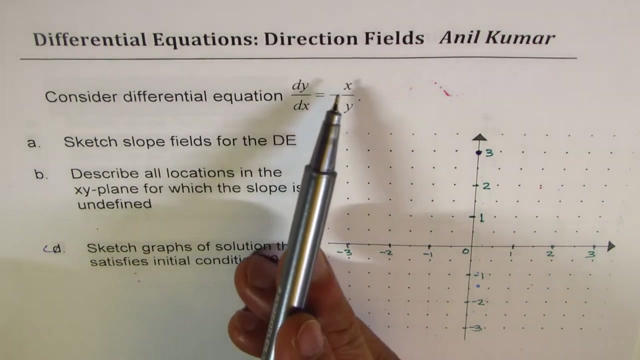 So we will sketch graphs of solution that satisfies the initial condition: zero three. So we will sketch a graph going through zero three, right? So that is what we have to do Now. here there are very interesting things. Before we get into sketching, let us try to analyze what we have. 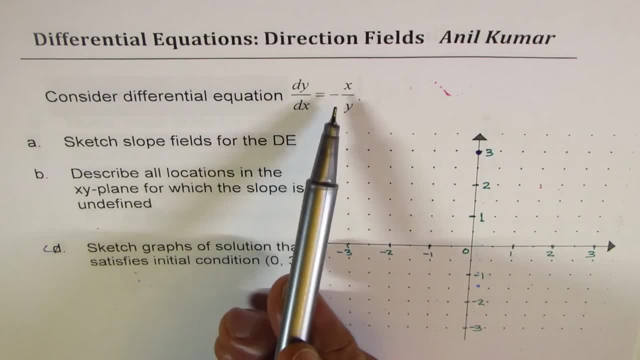 So we are saying that the derivative, which is a slope, is dependent on the function itself and at any point, x and y, The slope is given by Ratio of x and y, with a negative value. That is what we say here. Now I will just plot x and y values. 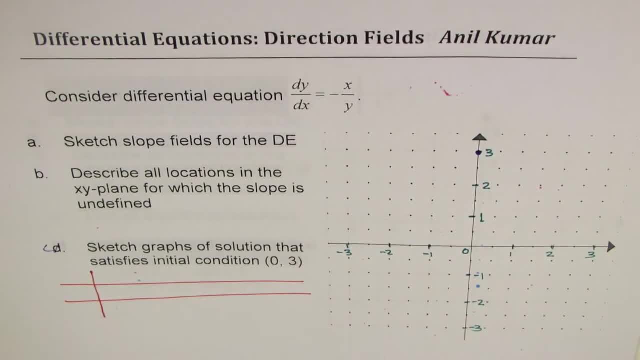 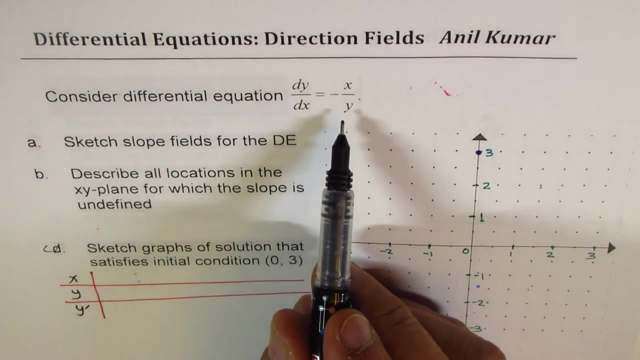 Let me do it horizontally this time. So what we will do here is that we will write x values, y values and the slope, Which is their ratio, with a negative sign. Is it okay? That is what we will do. So what do you observe? 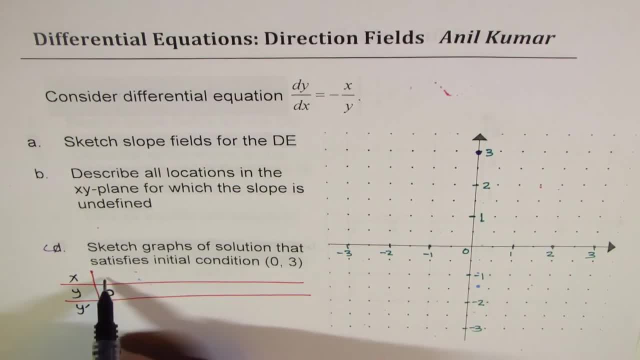 If I put y as zero, then what happens Then? for any value of x it does not exist. Do you see that part That is very important. If y is zero, that means along the x axis it does not exist. It means it is not defined, right? 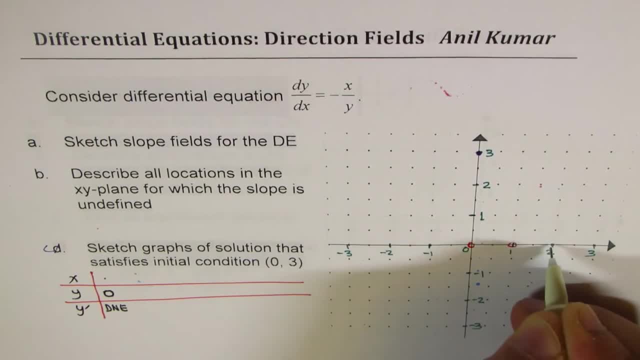 So I will make small holes here. All along this x axis, I am going to make some holes here. It only means that It is not defined. It is not defined, It is not defined at this point, Correct. So that is very important thing. 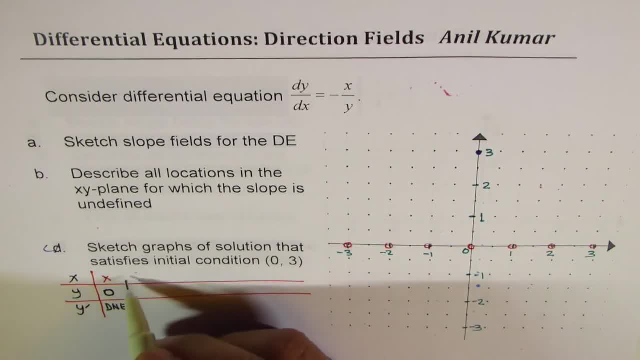 Now, what happens for any value of x? right, For any value of x. that is the scenario. Now, if I take the value of x as zero- Let us now take x as zero- Then of course we will consider all y's but not zero. 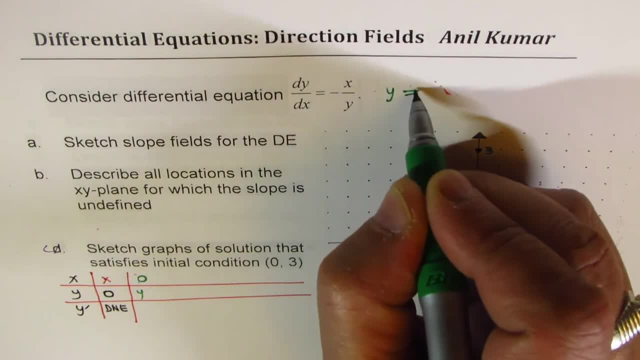 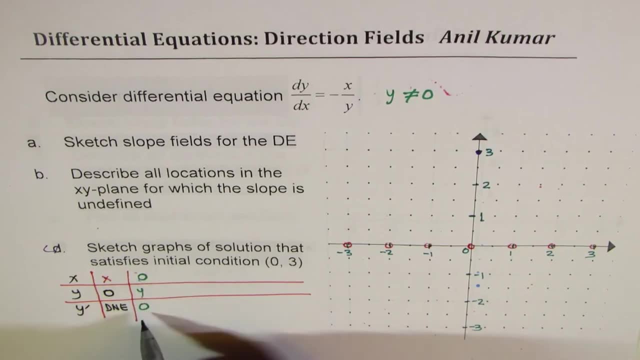 All y's but not zero. So we will write here that y is not equal to zero, Is it okay? It is not equal to zero, guys. In that case, the slope is going to be zero. That means horizontal, Is it okay? 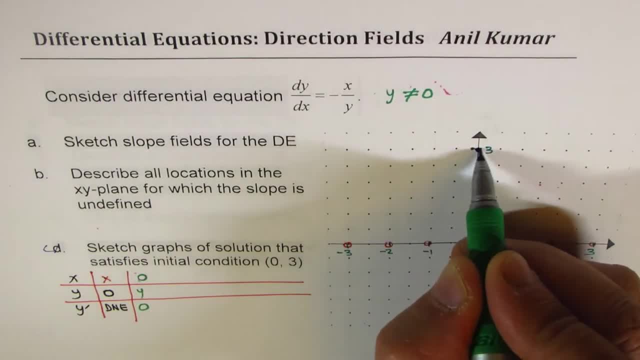 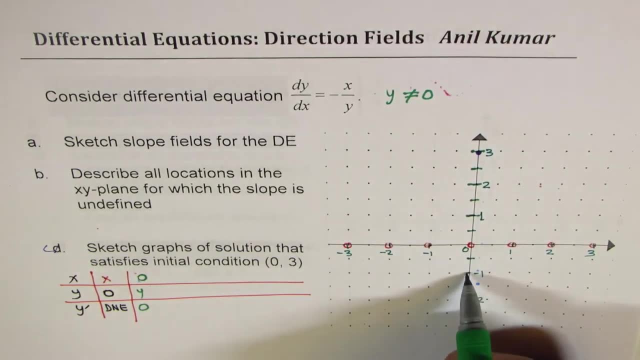 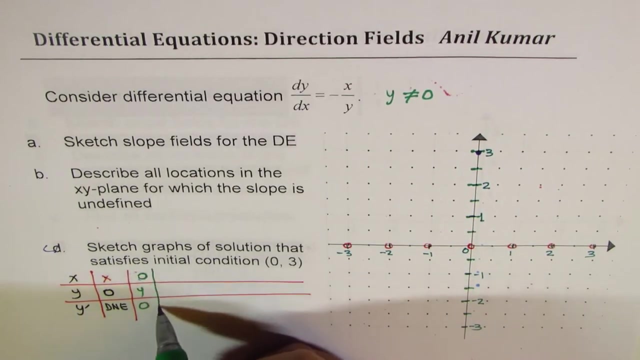 So whenever x is zero, it is horizontal. That means all along the y axis it is horizontal. Let me draw here also small segments At point five I am drawing. Okay, Fine, So we get the zero points. It is good to analyze. 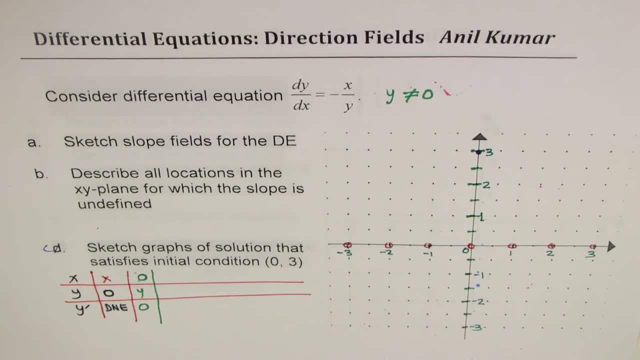 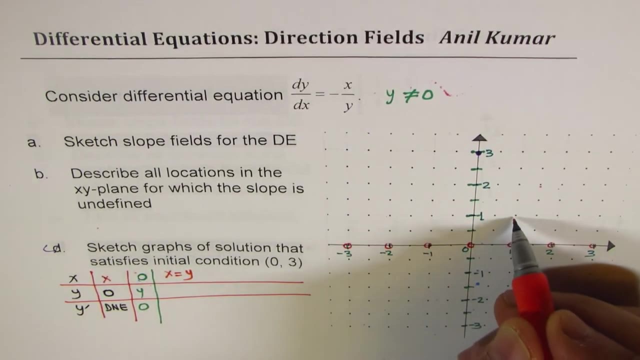 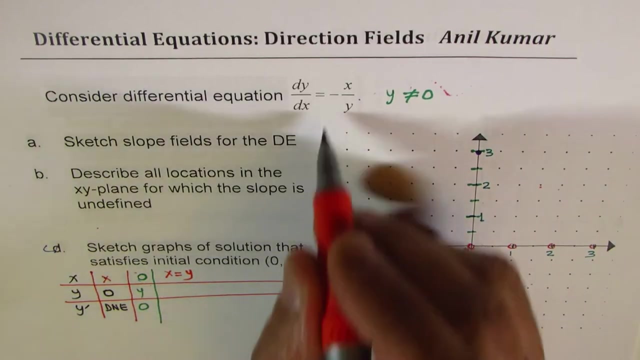 then substitute the points, otherwise this job becomes very tedious. now, if i take x equals to y, let us say x equals to y. so now i am considering the point where x is equal to y. that means points like 1, 1, 2, 2, 3, 3. then what happens if x is equals to y? right, in that case we get minus 1 here. 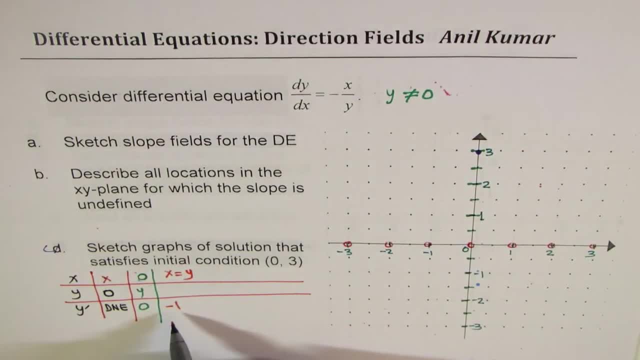 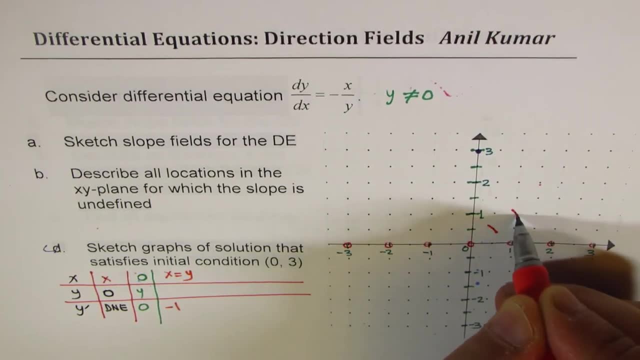 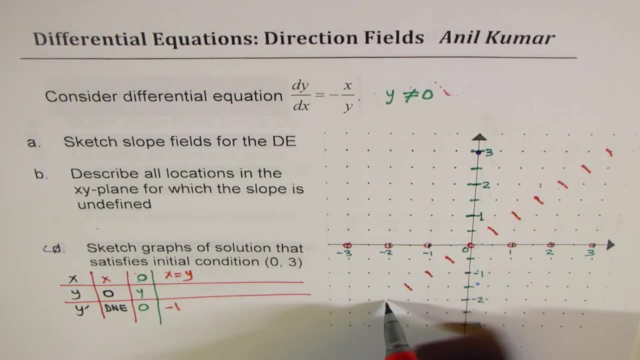 because they are same right. so slope is negative. 1. that means dropping down, so that means along this diagonal it is dropping down, so that becomes the slope along this diagonal. do you see that? so we'll not touch the x-axis. there it is not defined, but all of the places we could draw this. 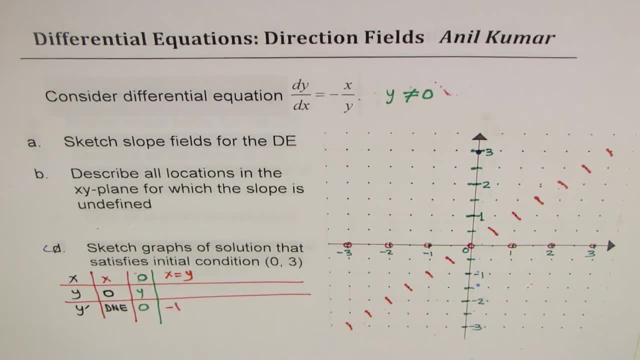 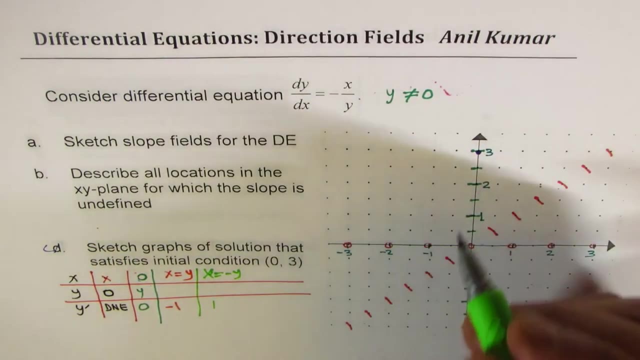 correct. now what happens if if x equals to minus y? if x equals to minus y, then we have plus 1 slope, right? so x equals to plus minus y means we are in quadrant 3 or in 4, right? so they are like negative of one another. so here it is going. 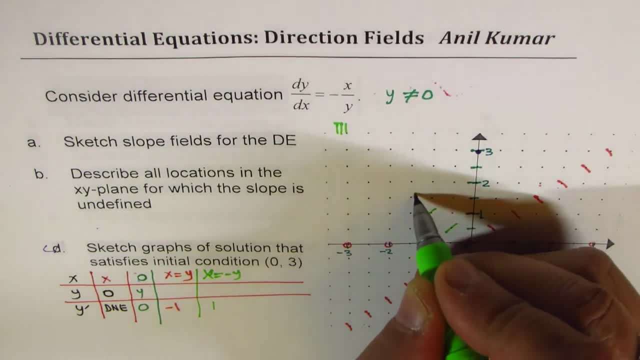 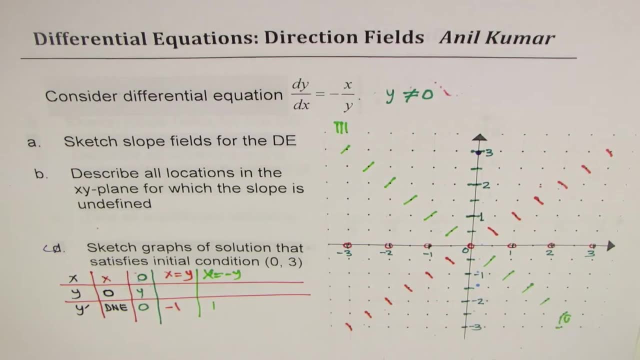 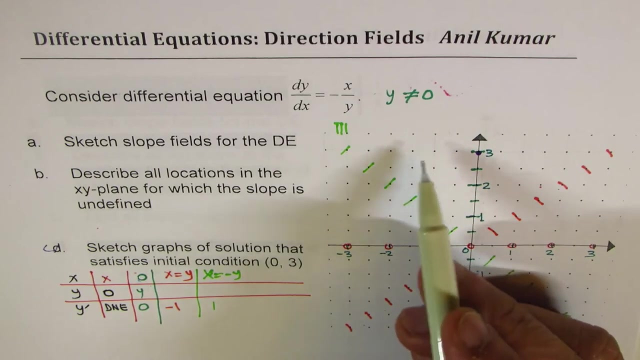 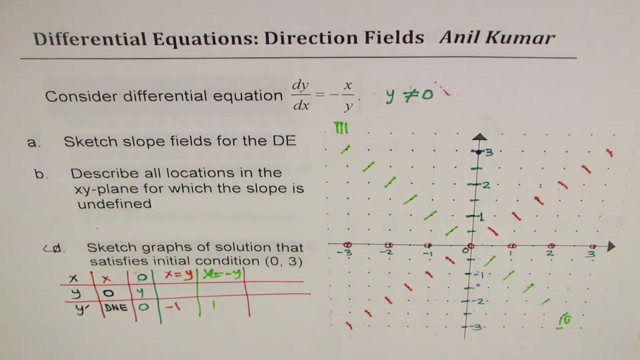 to be positive 1, so we could draw these as positive 1 slope, correct. so all these are positive 1, correct? now we can take some of the values for x and then draw, for example: now if i take x as minus 1, then for different values of y, what do we get? so if i take x as minus 1, let us say 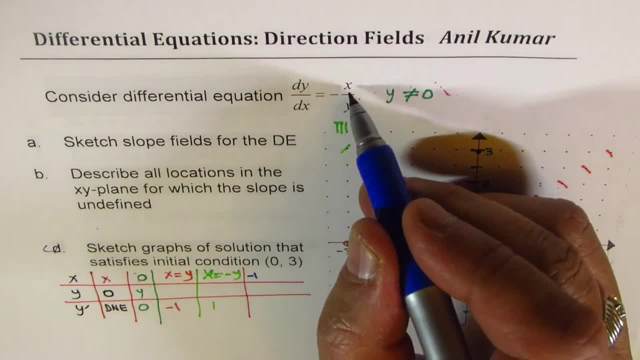 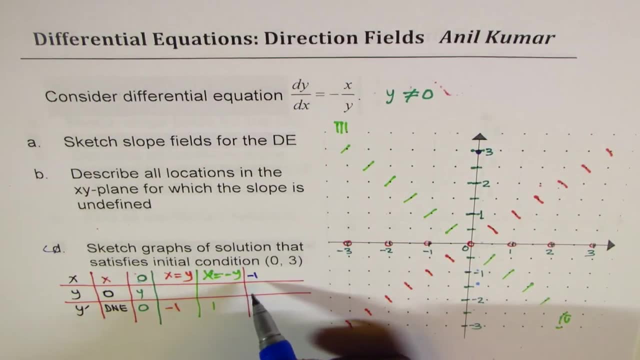 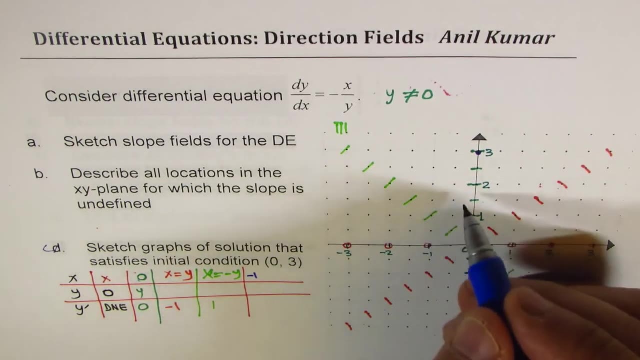 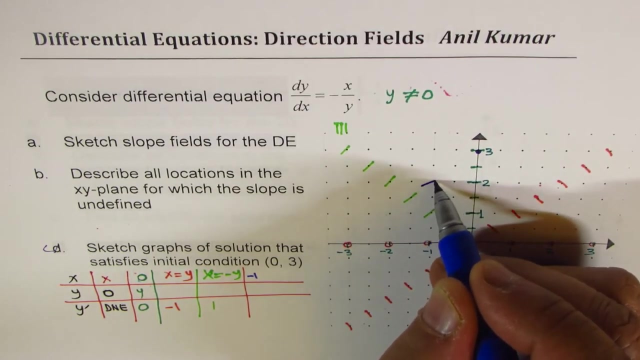 then this becomes positive reciprocal of y, correct? so so for minus 1, minus 1 and 1, we have already drawn. but if I take minus 1 and 2 then becomes half. that means lesser slope. do you see that it is lesser slope, kind of like? 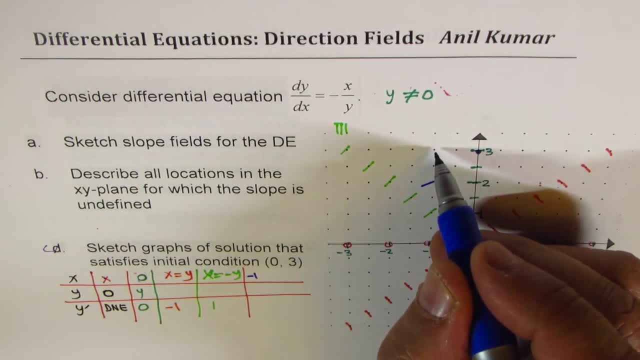 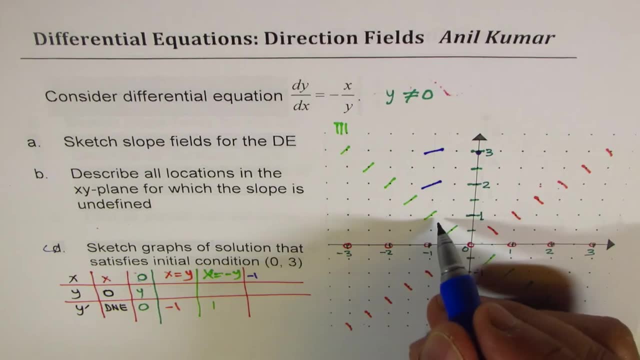 this. and if it is 1 over 3, then becomes even lesser, even less. do you get my point? but if it is less than 1, it means if I take half as a value, it becomes 2, so it is more slope. so that is what happens when Y value is positive. but if 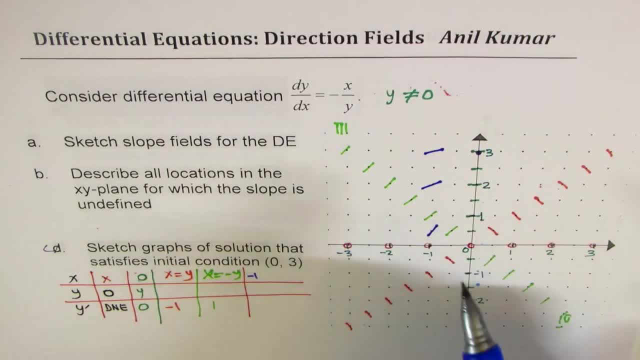 Y value is negative, then in that case it becomes negative. for half it becomes negative. 2 steeper Y for one we have already drawn negative, and if it is 2, then it becomes half less steep but negative. and if it's 3 it's less steep and it becomes half less steep but negative, and if it is 3 it is. 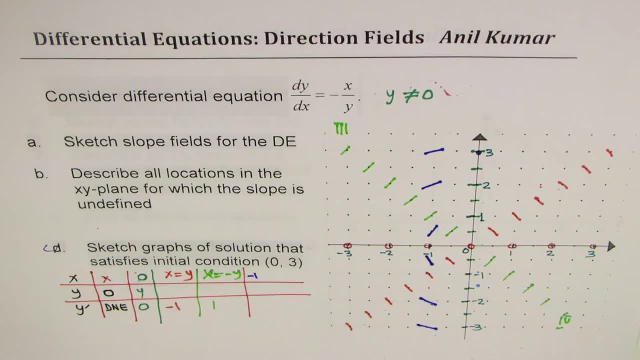 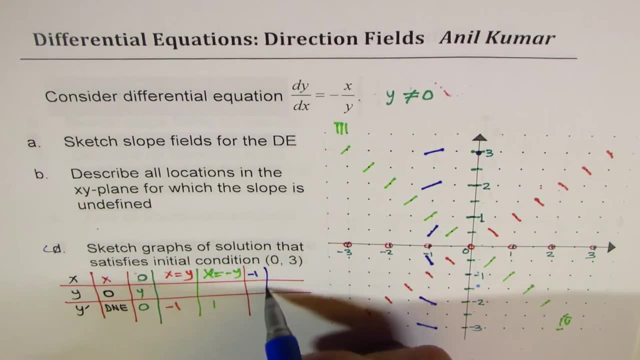 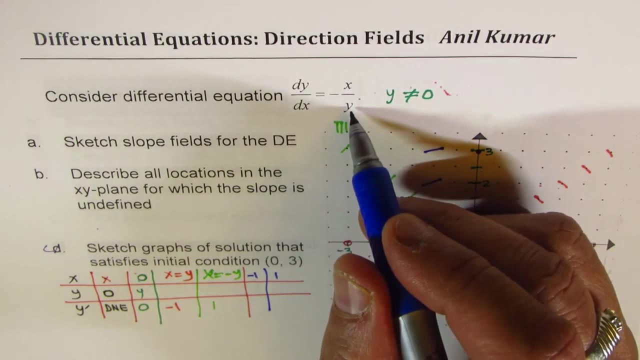 even less steeper right, So more towards horizontal. Do you see that? So that is how the slope will be if we look into this side Now. similarly, if I look at x equals 2 plus 1, then we are getting negative of y values. That is to say, if I take x as plus 1, that is along. 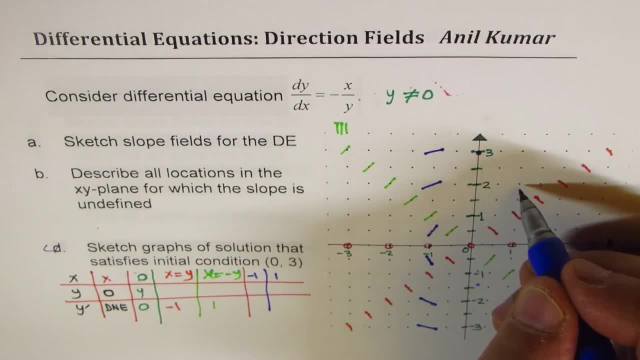 this line and y as 2, then we have negative 2 slope. So it is dropping down like this: Negative 2 is steep, right, I mean half, So less steep, So at minus 1, it is kind of like this, And with 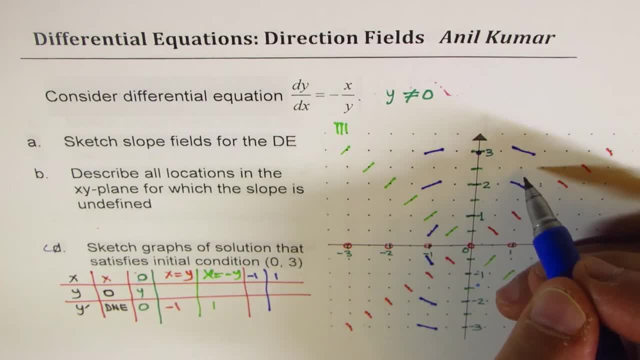 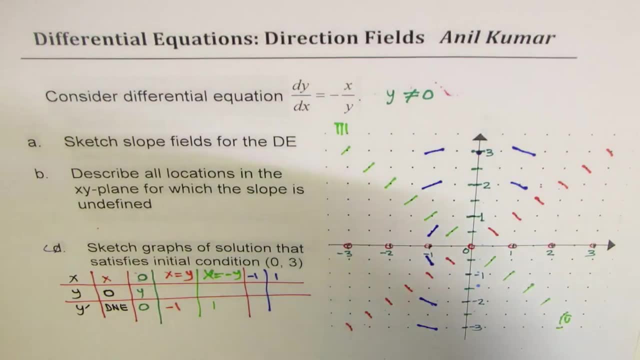 3, it is even less steep because it is one-third correct. So it is negative up to here. But as soon as the y value becomes negative, it makes that positive, So it becomes positive. slope and denominator increases. slope decreases and becomes more and more horizontal. Do you get the? 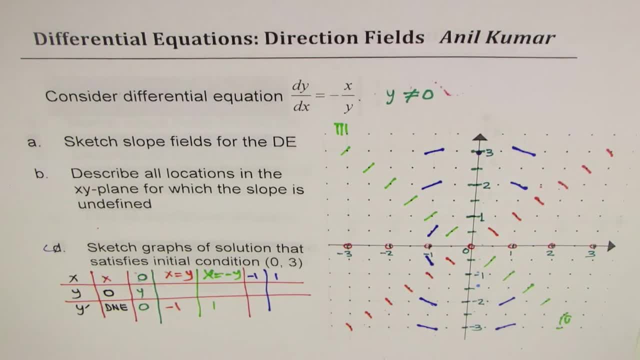 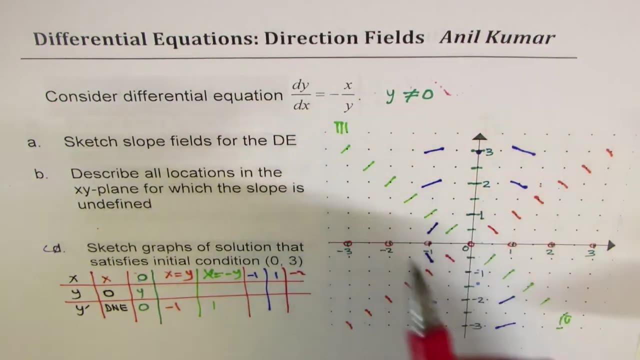 idea Correct. Now let us take a value of x which is minus 2. So we are just moving away now. So at minus 2,, that becomes minus 2.. Minus minus becomes positive, And now we get 2 over 1.. So 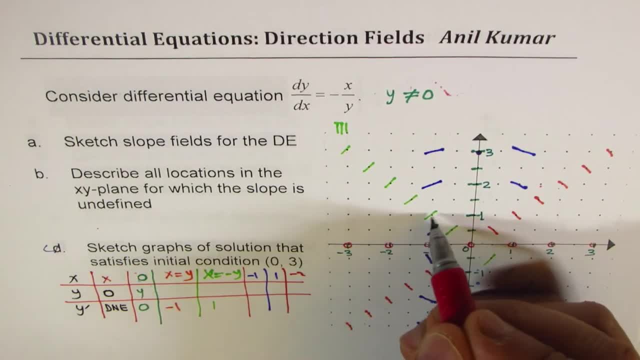 the slope here is 2 over 1.. So twice this, Twice this. So it is steeper than this 2 over 1.. So it is twice what we had there. Do you see that? It is twice that we have there, So we could just make slightly. 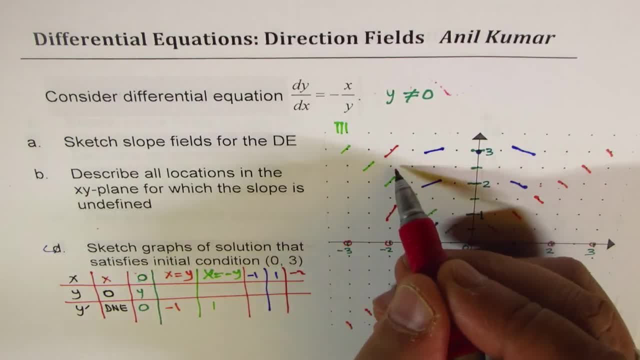 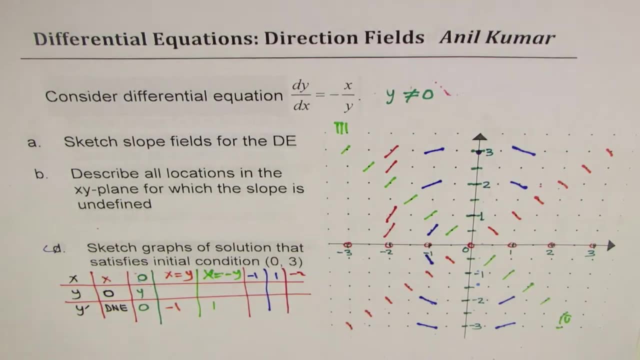 more steeper than this point? Do you get my idea right? So it is slightly more steeper than this. That is what we are trying to say, Correct? If the y value is negative, then negative y is negative, So negative y is negative, So negative y is negative, So negative y is. 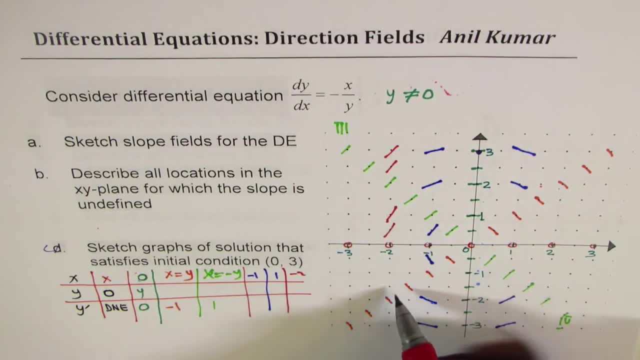 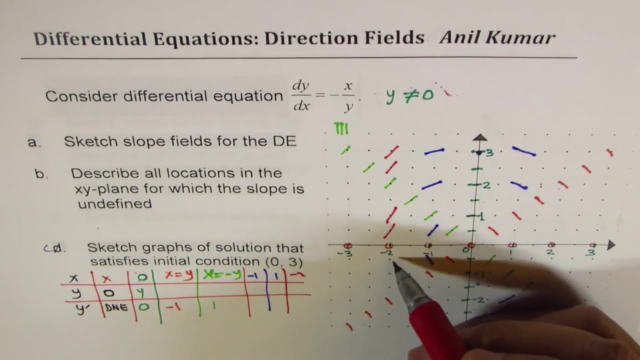 negative, It makes this one also negative. So here, all the slopes are going to be negative, Perfect, All slopes are dropping down And minus 2 over. minus 1 is going to be is just 1, right. So at this point it is going to be minus 2 and minus 1 is going to be minus 2.. 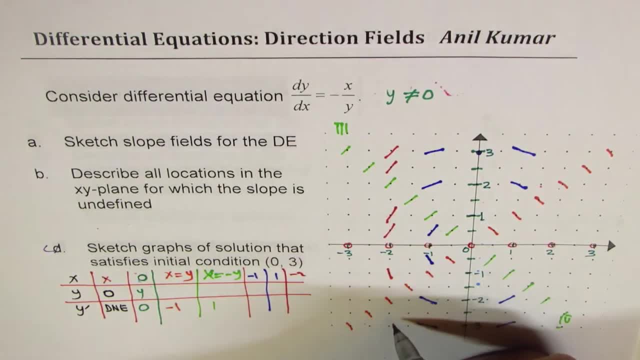 So it will be steeper than this minus 2.. And as we go further down, y value increases, so it becomes more horizontal. You get an idea. So what do you see? here is kind of a circle. Do you see the pattern here? Kind of a circle. So that is what we observe. Now let us take 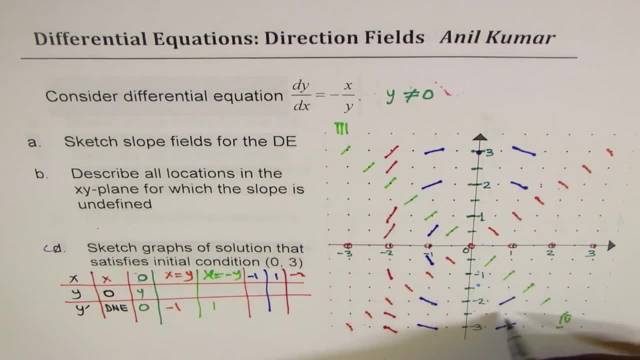 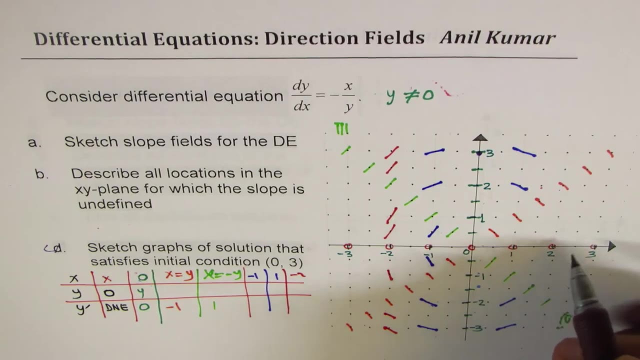 few more points and then we can draw our patterns. You can already see the pattern here, which is kind of circular, right? So let us move on and take some more points. So if I take x as plus 2, now we have already taken 1.. If I take plus 2, we have a negative value for y, positive. So 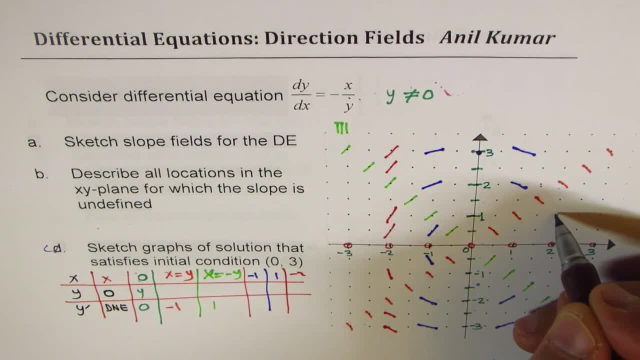 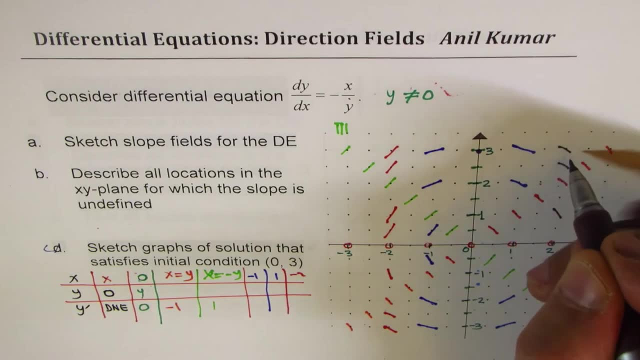 if y is 1, the slope is 2, negative 2, right, So it is kind of negative 2.. As the y increases, the slope decreases, So it becomes kind of flatter. Do you see that? So that is how it is. 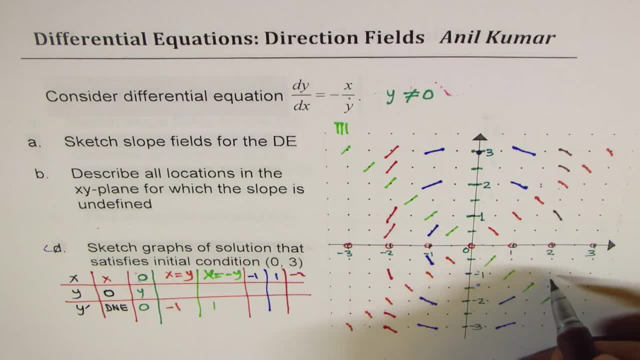 On the right side when we go down slope is 2 divided by 1, minus, minus. minus becomes plus. so it is positive. So it is positive here, but as we go down it becomes lesser and lesser steep. 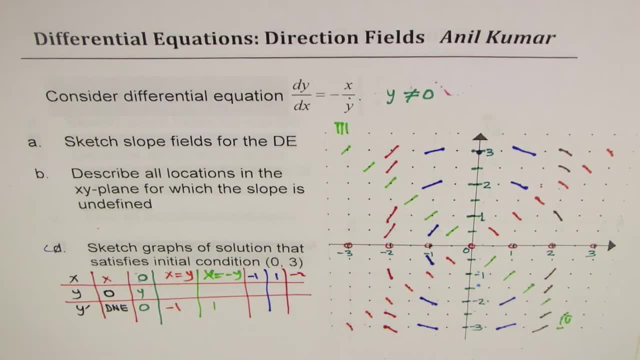 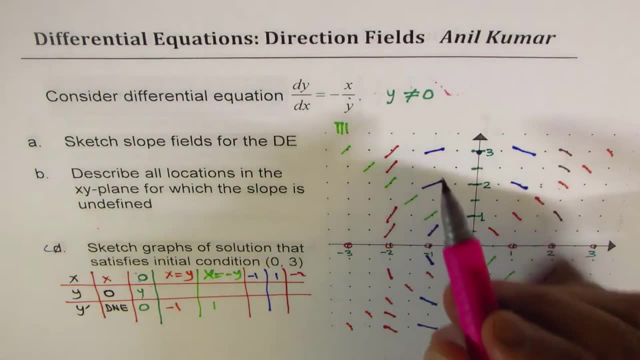 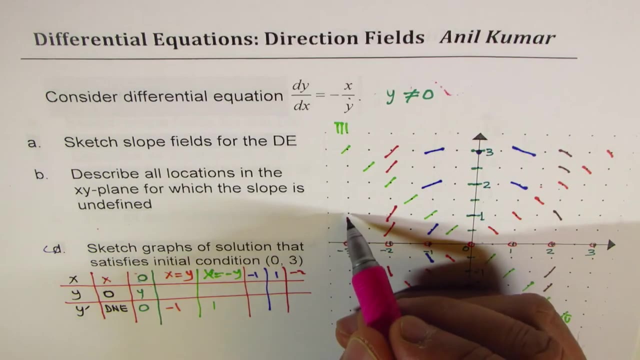 correct. Similarly, if I take the value of x as, let us say now, 3, minus right. So minus and minus becomes positive. as the value of y is 1, it is minus 3, that means coming down. Sorry, minus and minus is positive, so positive. 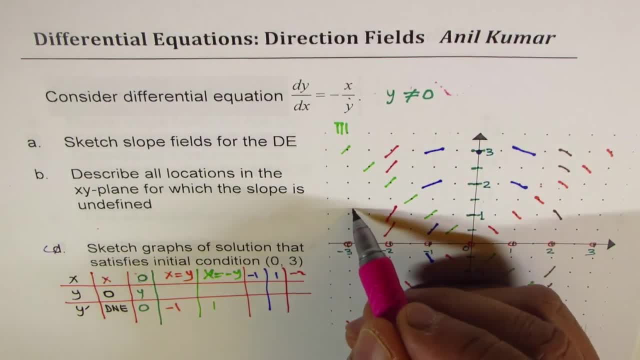 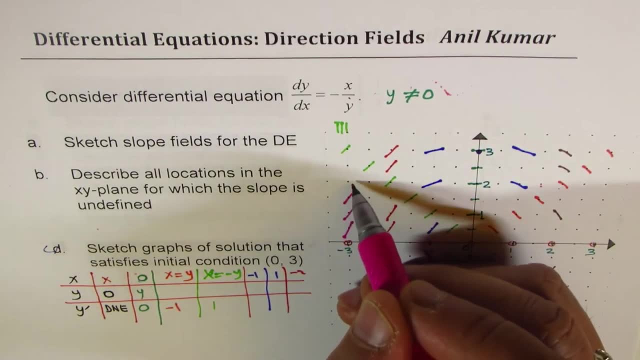 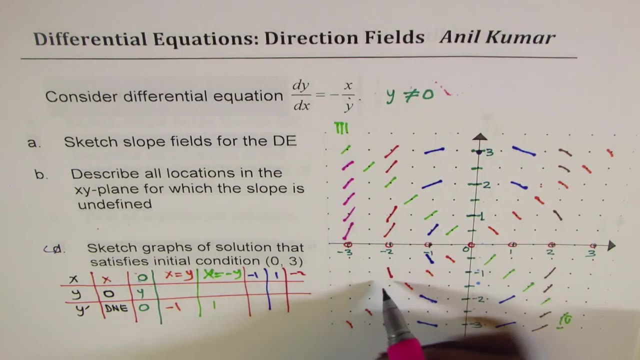 3 for y equals to 1.. So steep, positive, 3. As y value decreases, it becomes steeper, and if y value increases, it becomes less and less steep. correct Now on this side: since y is negative, slope becomes for negative. 3, positive becomes negative, So we have negative. 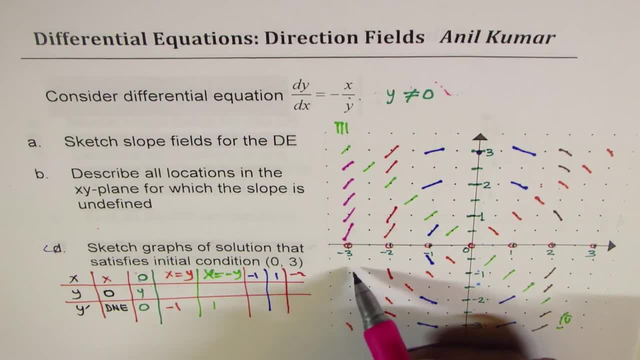 slope here and as we go down it becomes lesser and lesser steep, right? So here it is more steep and then it becomes lesser and lesser steep. So what do you see here is kind of a circular pattern. So that is how you can actually fill this up and see very clearly what we are going to. 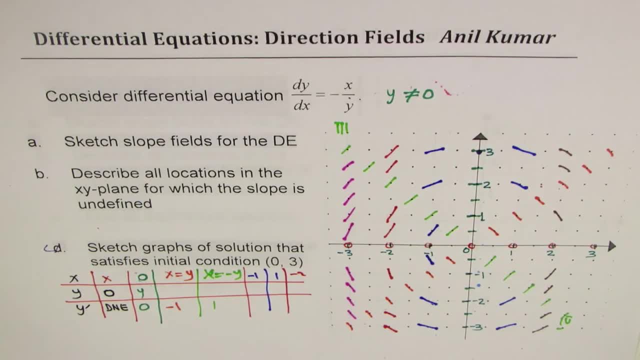 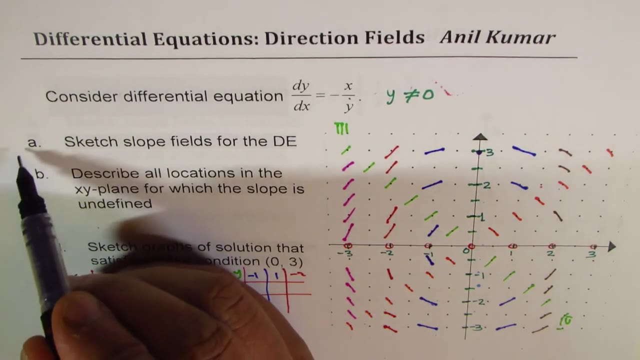 get right. So slope fields- again I want to emphasize- gives you a geometrical look of the solution So you can appreciate how the solution will look like. Now let us get to the part B. now We have done part A, that is, 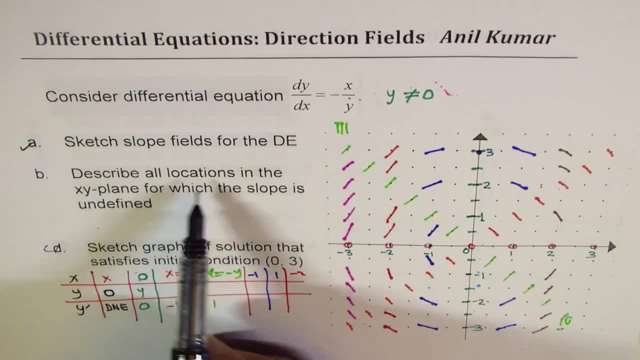 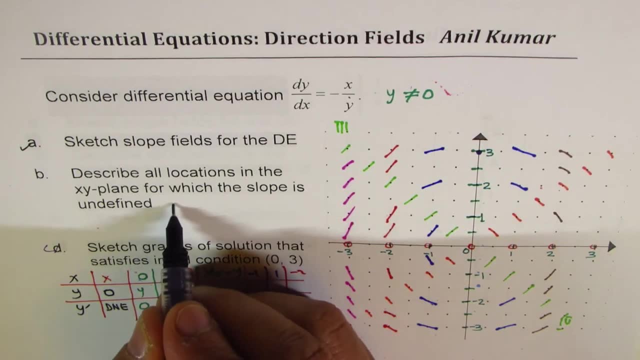 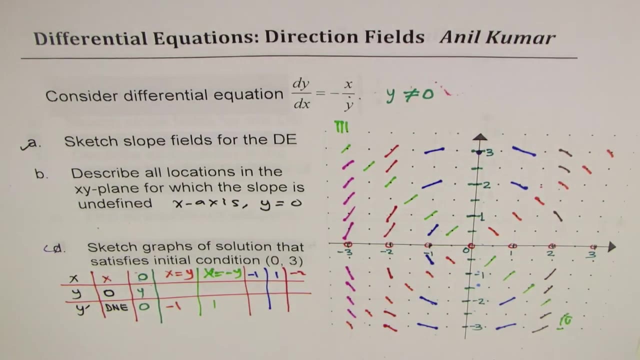 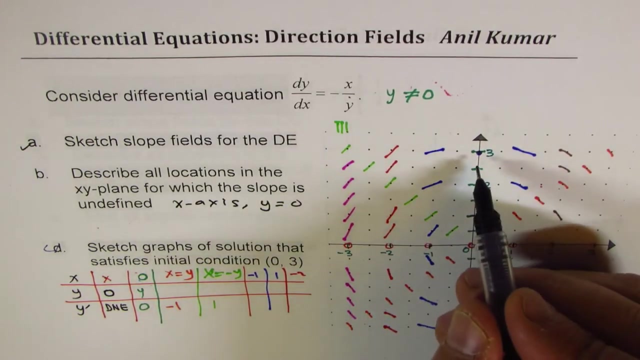 sketching the slope fields Describe all locations in the xy plane for which the slope is undefined. So it is undefined for x-axis where y is equal to 0,. right, We just filled that up with holes here. C sketch the graph of the solution that satisfies initial condition 0, 3.. Now 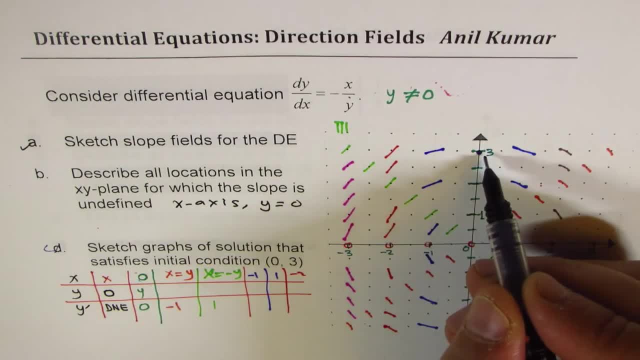 if I have to draw a graph here, then it should go like tangential to all the points which we have drawn, correct? So we have some fields here. You could have packed this up also. So, starting from here on the left side, we can see that the graph goes. 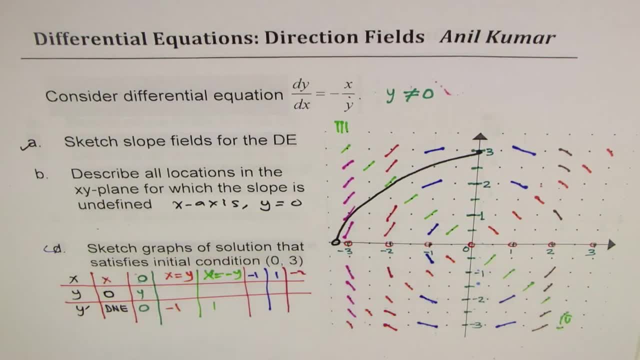 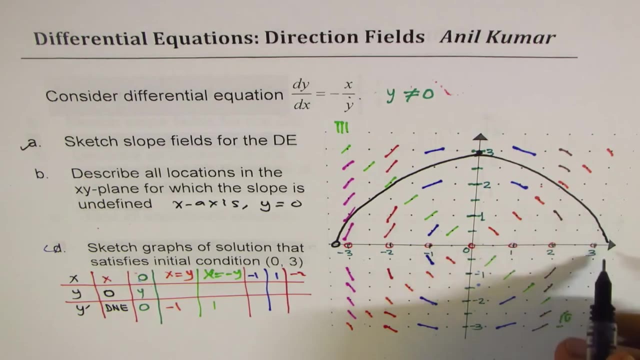 like this, but we have to stop here, since that on x-axis it is undefined. Do you see that part? So that is very important to understand. So, similarly, on the right side also, it is going to be kind of like this, but as soon as you approach this, it becomes steeper. 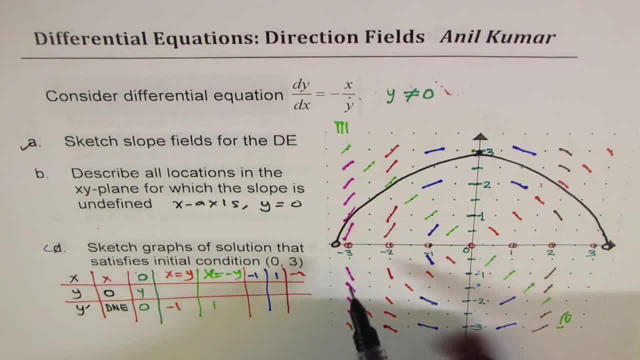 you stop here. You should not be crossing it. Some students can do a mistake by continuing this and making kind of an ellipse or a circle whatever, but then if you do that it is not a function. It will fail the vertical line test. So I hope it is very important to understand. 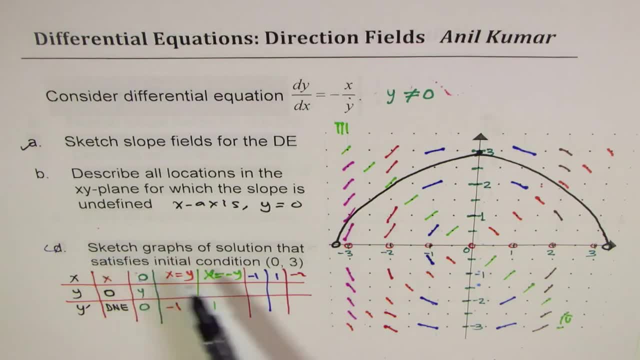 that for different values, different initial values, we will have different solutions. These are called particular solutions based on initial values In general. you may see that it represents kind of a circle, right? So we will actually take this up in more details later and see what it really represents. 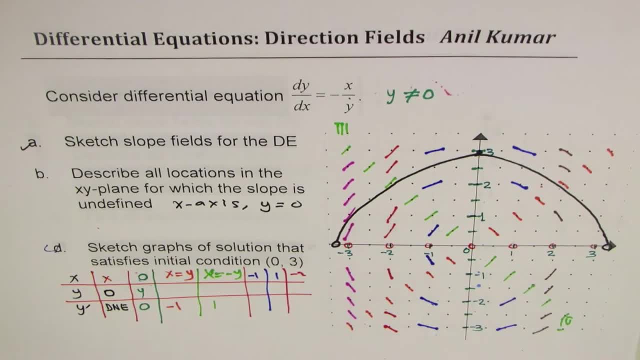 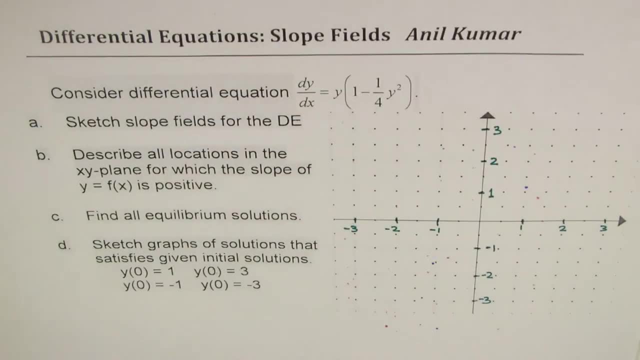 but I hope with that you get a fairly good idea of how to sketch slope fields and how to interpret the solution of a differential equation correct. So let us now. we are almost at the end and here is the final question for you. With all the information you have, I would like you to 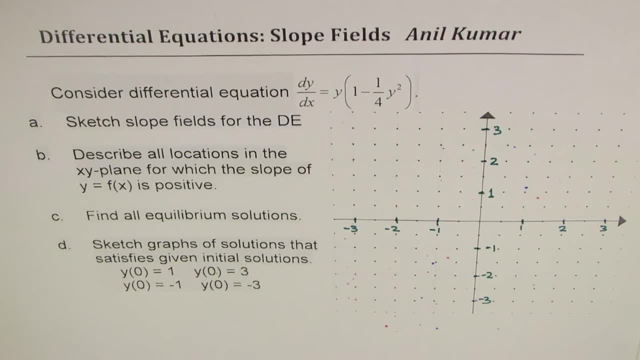 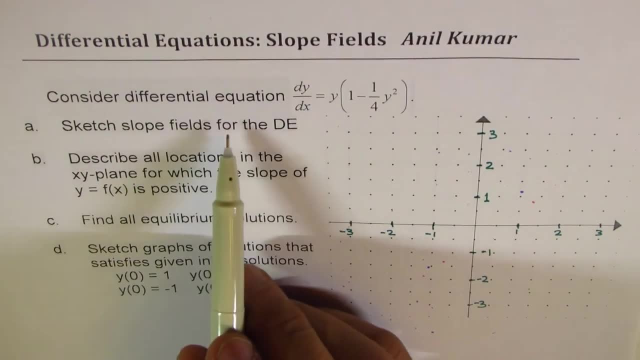 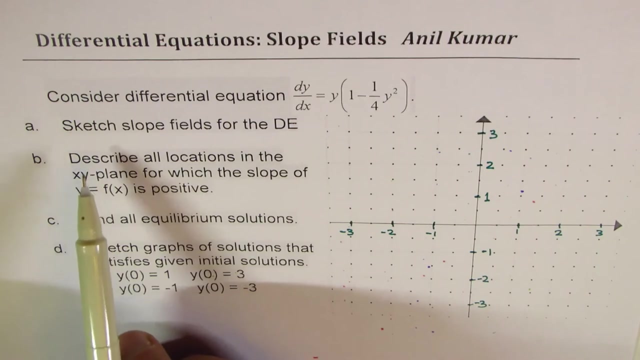 pause the video now, copy the question sketch and then see my suggestions. Now let us consider the differential equation. divide dx equals to y times 1 minus 1 over 4 y square. We need to sketch slope fields for the differential equation, describe all locations. 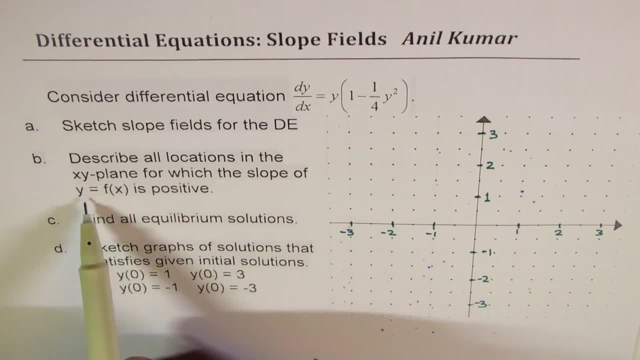 in the xy plane for which the slope of y equals to f, of x is positive. C is find all equilibrium solutions and D is sketch graphs of solutions that satisfies given initial condition, y0 equals to 1.. So these are different conditions. right: y0 equals to 1,. 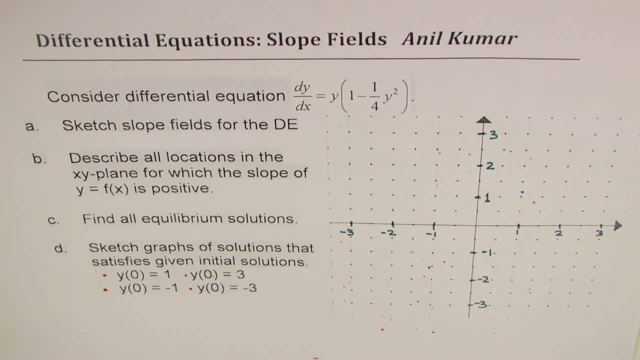 y0 equals to 3, y0 equals to minus 1, y0 equals to minus 3.. That means we are looking for four graphs, right, Four initial solutions, right. So now, what we have learned here is also how to quickly sketch slope fields. These are short dashes which 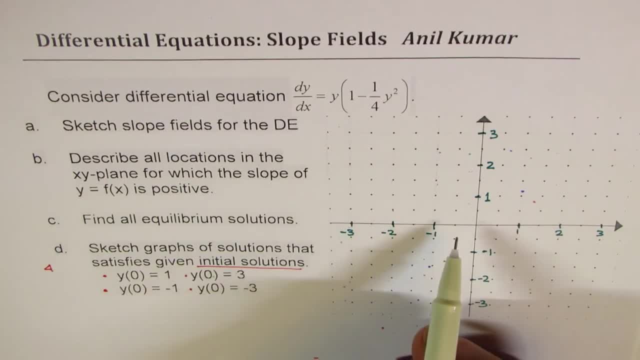 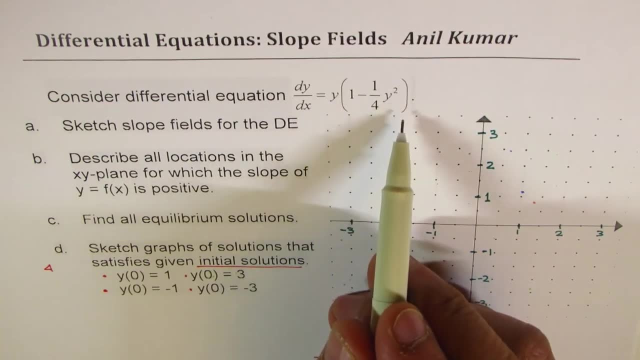 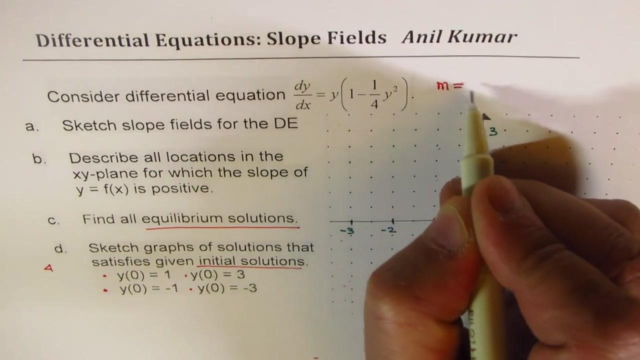 represent slope at any point on the Cartesian plane. We are given differential equation. divide dx equals to y times all this. Now let us find where do we get equilibrium solutions right? So when we say equilibrium solutions, we want to say slope is 0.. Now clearly from here. 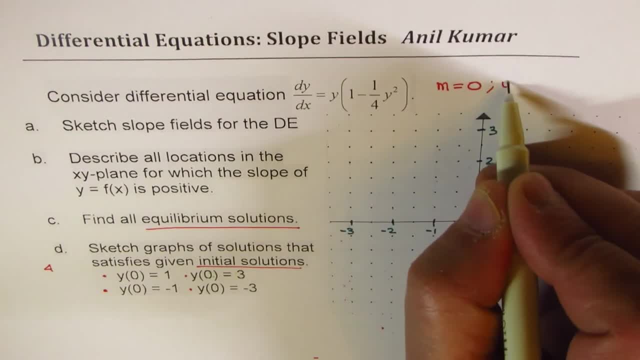 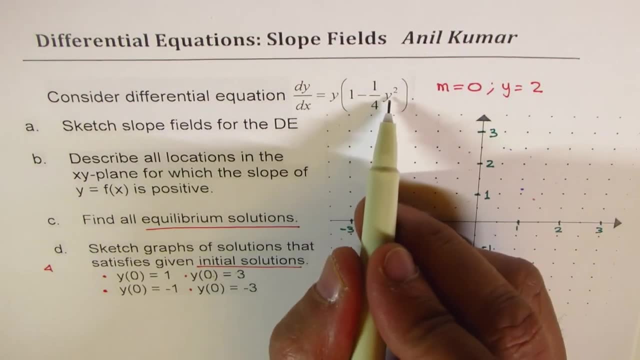 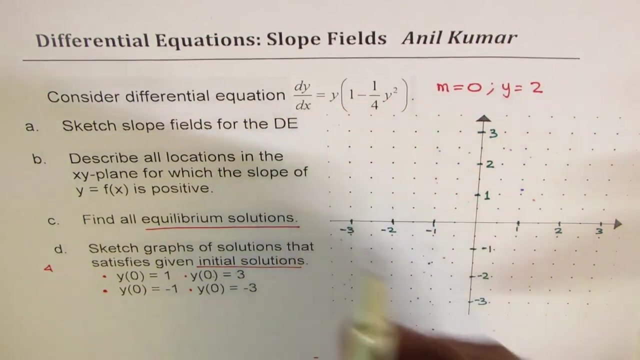 we have a solution for y equals to 2, right. So 1 is at y equals to. I mean y equals to 2 will give me 1 minus 1.. I mean if I write 2 here, y square is 4, 4 divided by 4 is 1.. So 1 minus 1 is 0, and 1 is y equals to 0.. 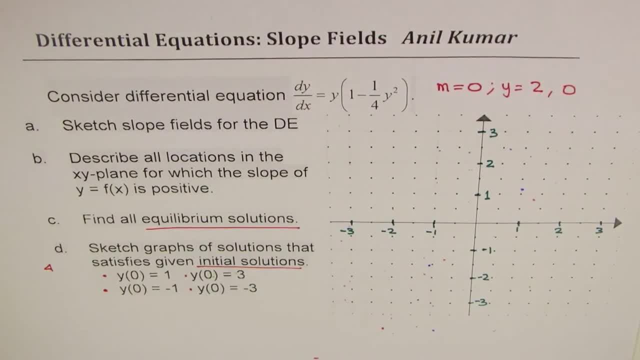 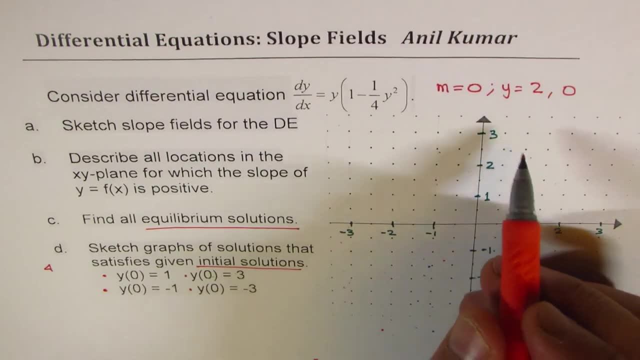 So these are two solutions which are equilibrium solutions. Now, at these points, we will have a solution for y equals to 2.. So we will have a solution for y equals to 2.. So we will have a solution for y equals to 2.. 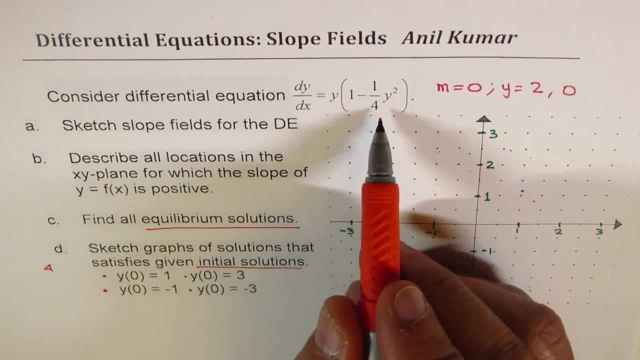 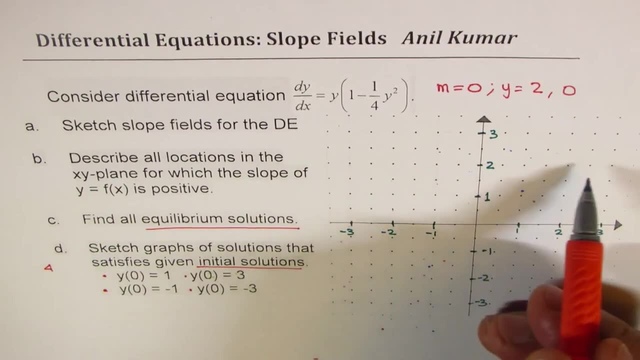 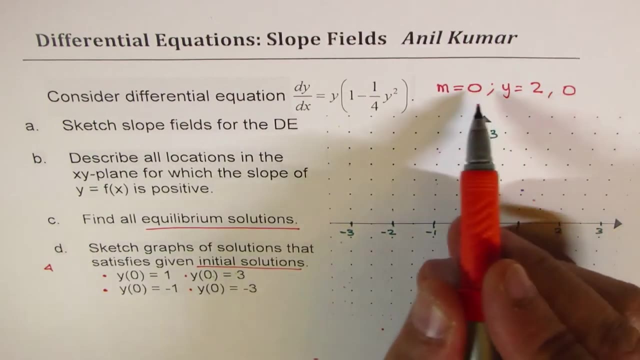 As you can see, the given differential equation solution is independent of x. So that means, like our first example, all along the y equals to this value, we will have the same slope right, So we can draw horizontal dashes along y equals to 2 and y equals to 0. So let us do that. 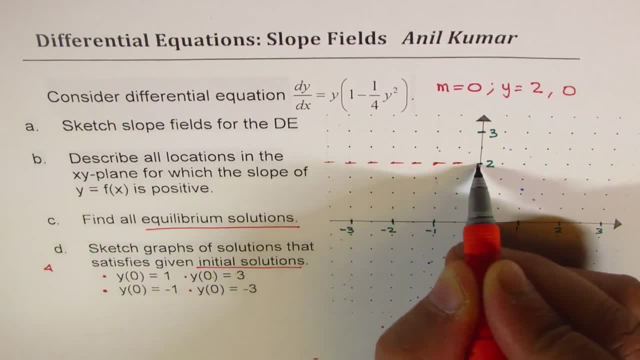 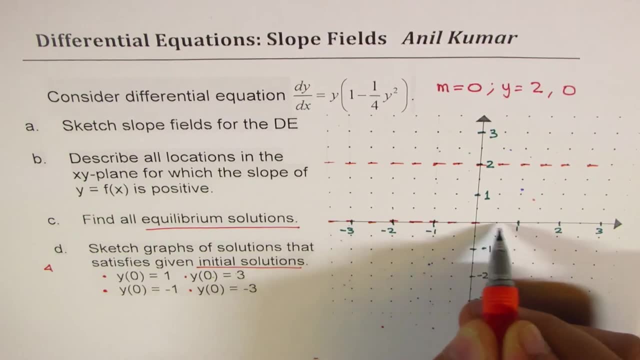 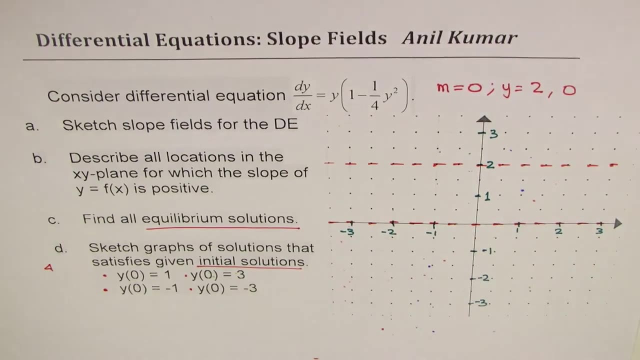 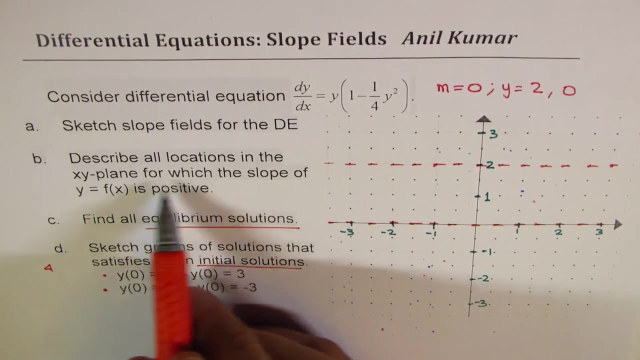 first part, And that is also the equilibrium solution for the given equation, right? So this is the. these are horizontals drawn as a part of our slope fields. Okay, Now we also want to know: when is this slope field positive? So when I say positive, then it means what? 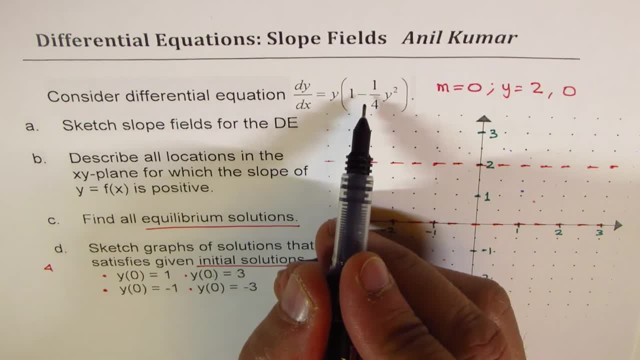 Why There are two factors, correct? So it is going to be positive when both are positive, or both are positive, So it is going to be positive when both are positive. So it is going to be positive when both are negative. correct? So there could be two conditions. So we are trying to answer this. 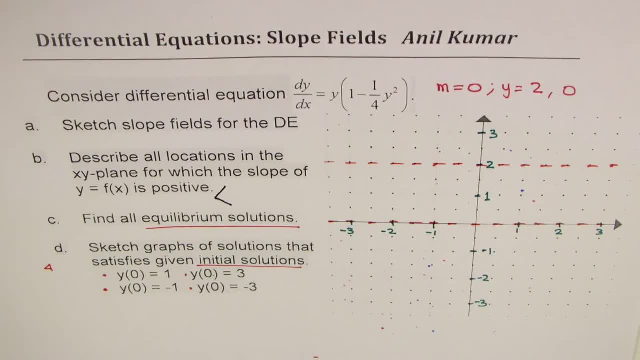 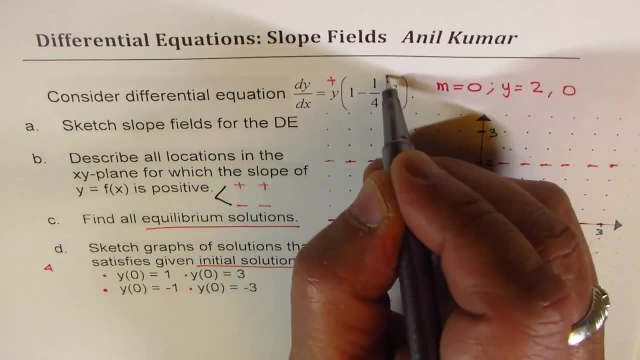 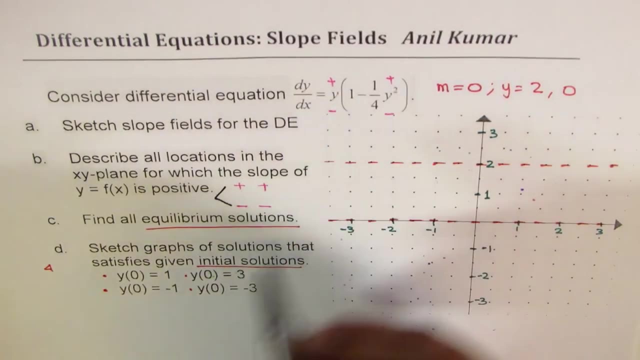 So there could be two conditions, that is, when we multiply positive with positive or we do negative times negative. That means this is positive, this is positive, or this is negative, this is negative. correct What I mean to say? these two factors. So when y is positive, 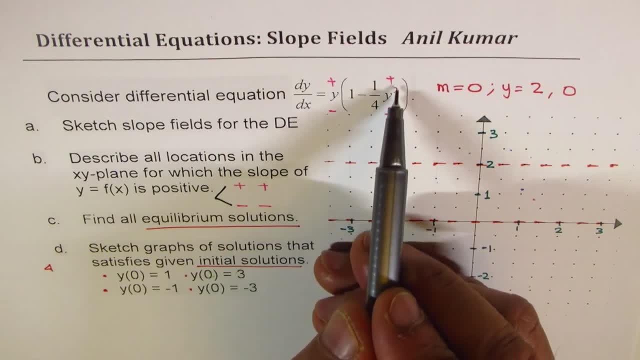 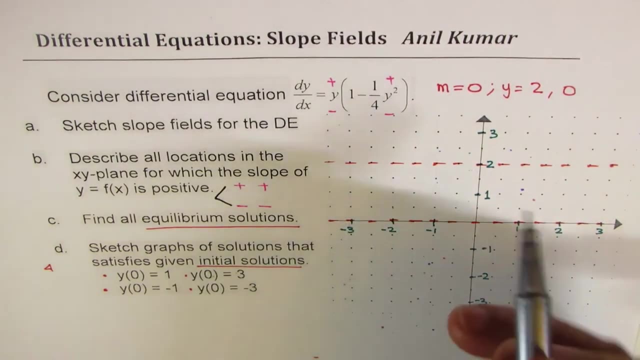 that means when we are looking at the upper half, when is the inside function positive? That is to say, if I write y equals to 2, then it is 0, right, 1 minus. if y value is less than 2, then this is positive. So in this period, 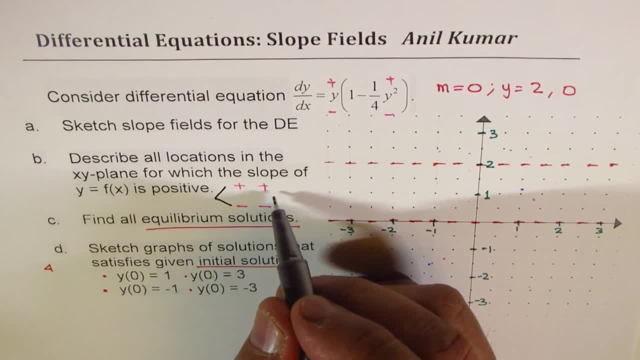 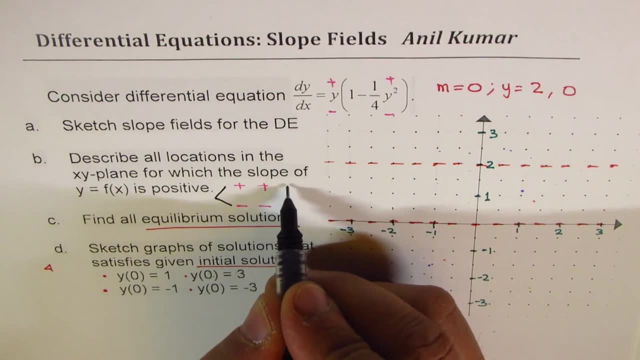 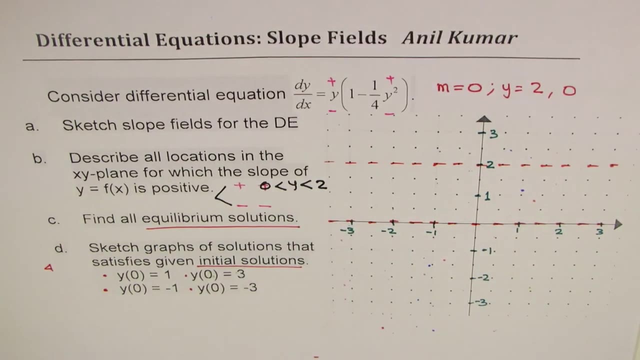 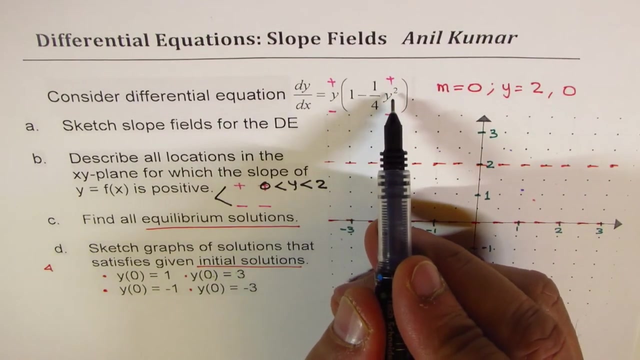 it is positive, correct? So the function is positive when y is between, when y is greater than 0,, 0 and is less than 2, correct? It is positive. Similarly, on the negative side, when both are negative. when is this negative? Now, y squared, that term will be negative if it is more than. 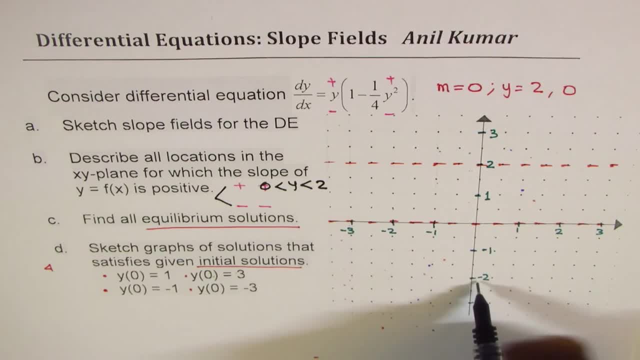 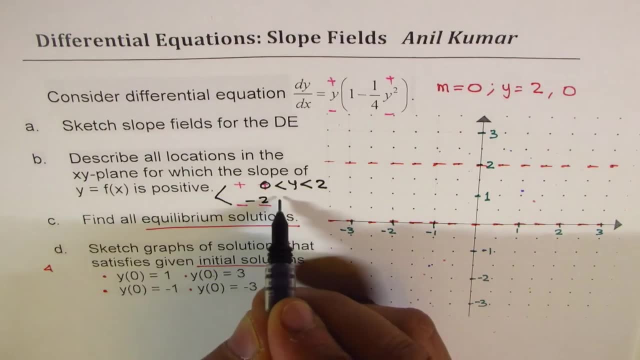 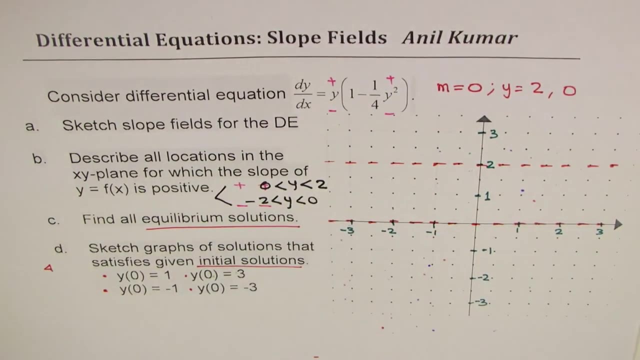 minus 2.. So if it is more than minus 2,, then it is negative. Does it make sense to you, right? So minus 2, I meant absolute value, because y is square right And it is between minus 2 and 0. That, even for y, equals to minus 2, we get a 0.. 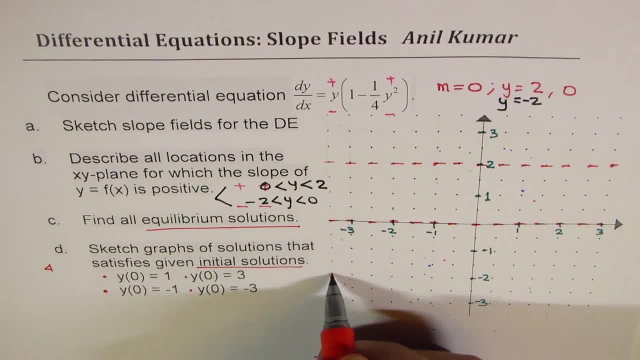 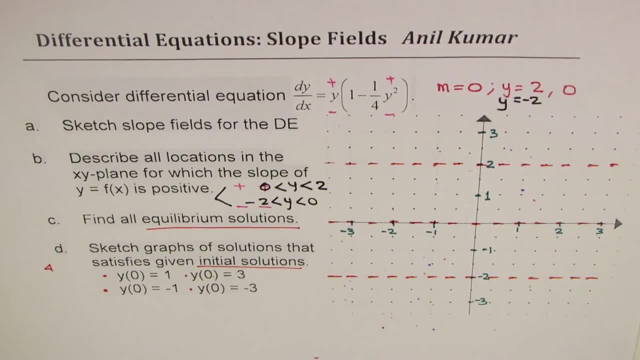 Is it okay. So I missed that part earlier. Here also it should have been 0s correct, Since it is y squared, so we get 0s here also. I should have sorry When y is less than minus 2,. 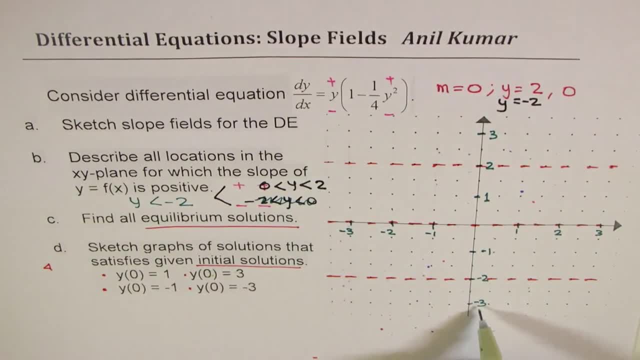 when it is on this side, then this is negative. Let us, if I put minus 3 here, if I put minus 3 here, in that case this is negative and minus 3 will make that as negative. So both becomes negative, right, So it is negative. here I mean negative. 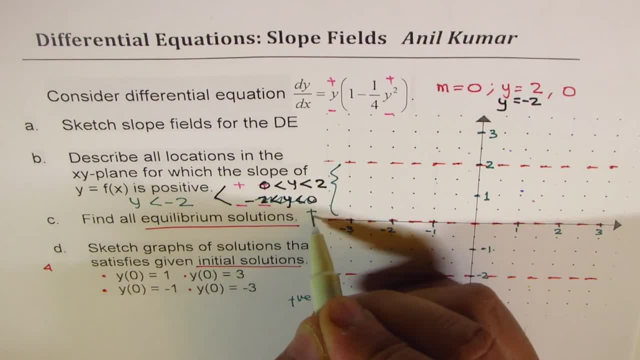 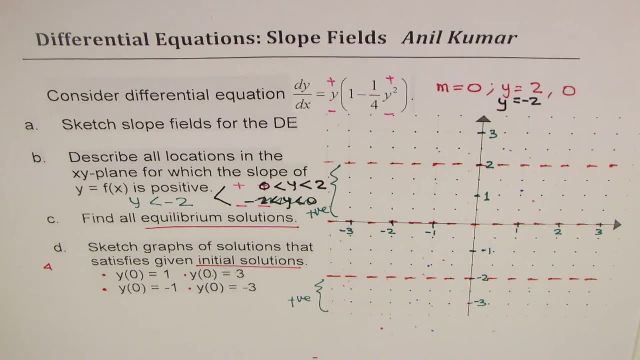 negative makes it positive. positive here and positive here, correct? So in these two portions it is going to be positive. In rest of the portions it is going to be negative. That is one part. Now let us sketch the slope fields. 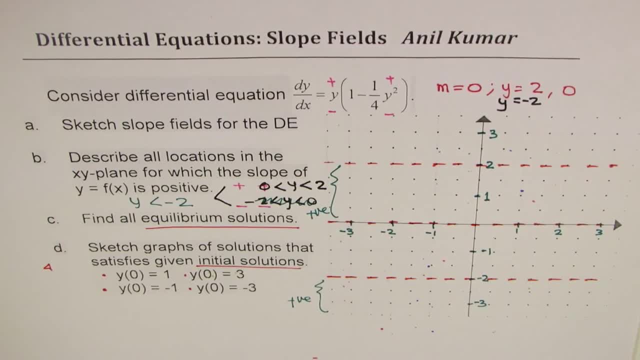 values of y, since we know that it is independent of x. correct? It is independent of x. So we will take different values of y and then we will write down the slope fields. Calculation is to be done based on this, correct? So if I take a value of y as 1, so we will write. 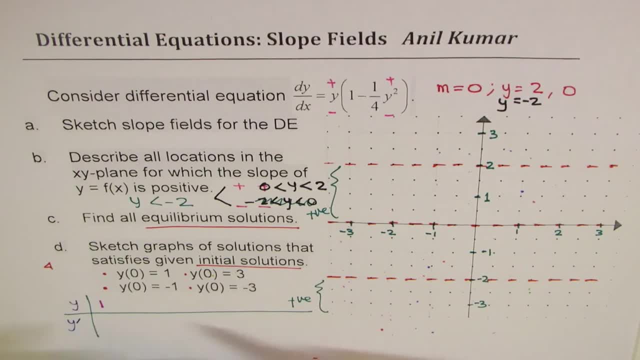 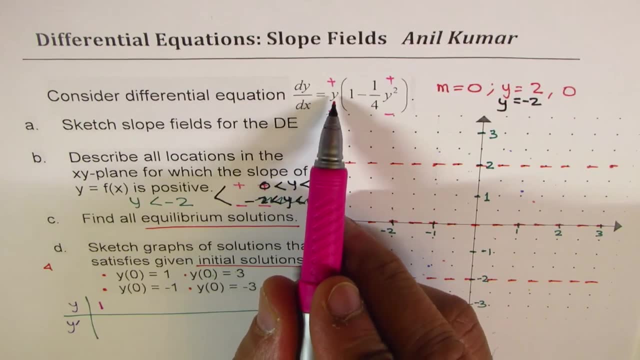 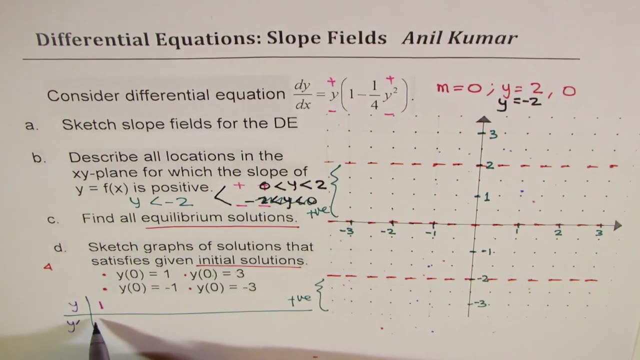 the y values here and we will write the derivative values or the slope underneath. So if I take y as 1,, in that case it will be 1, 1 minus 1 over 4.. That means 4 minus 1, 3 over 4.. So the slope is: 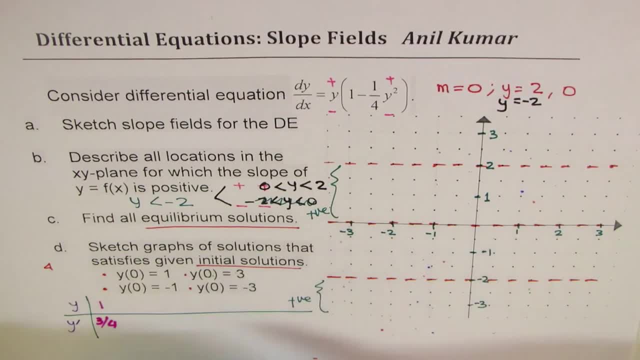 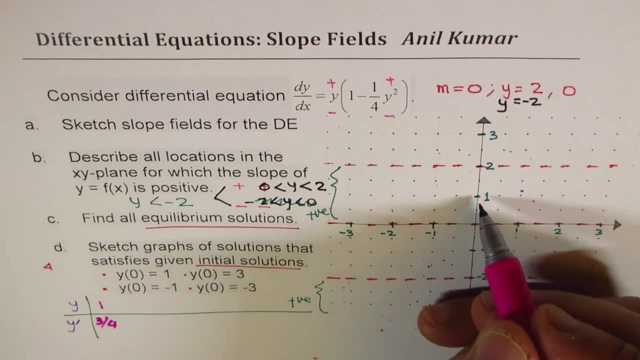 three-fourths right, So slightly less than 1.. So wherever y value is 1, the slope is three-fourth and it is positive as expected. So y value is 1 along this line. So three-fourth is less than 1.. 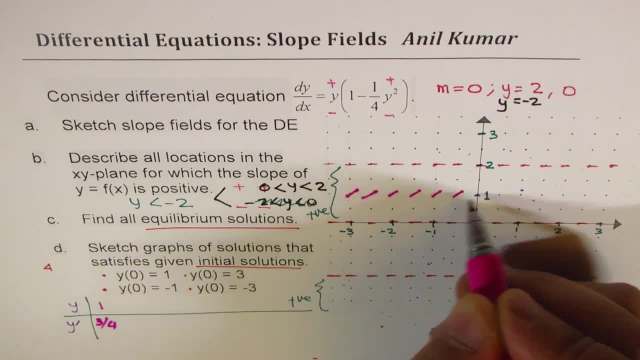 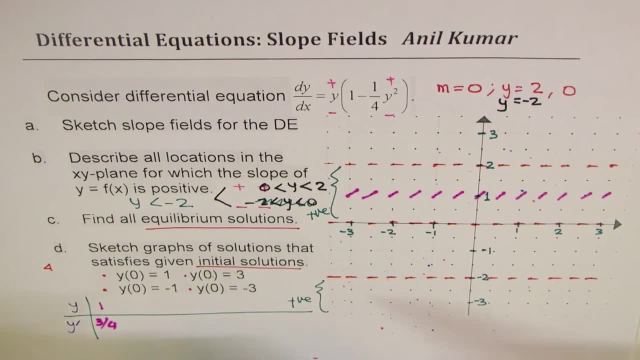 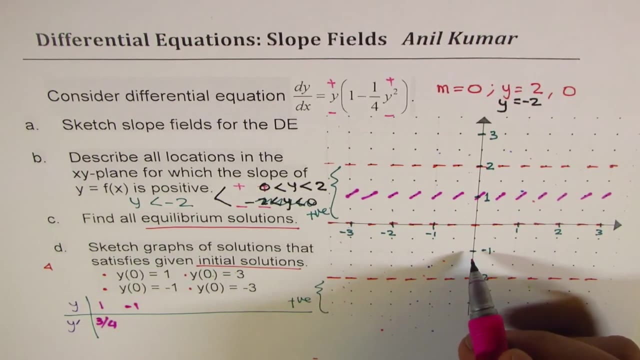 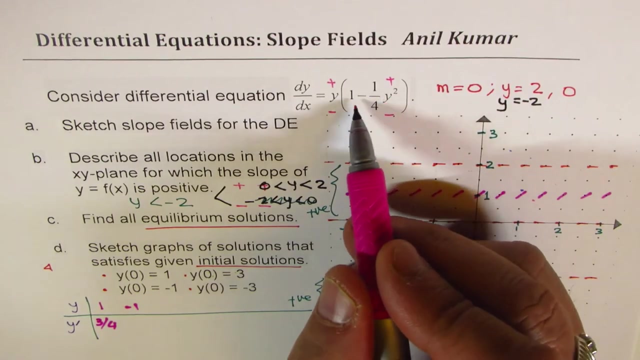 Draw these lines here as three-fourth slope correct. If I take minus 1, y value at minus 1, then what happens? So this still, this is again minus of 1. plus 1 does make this three-fourth. 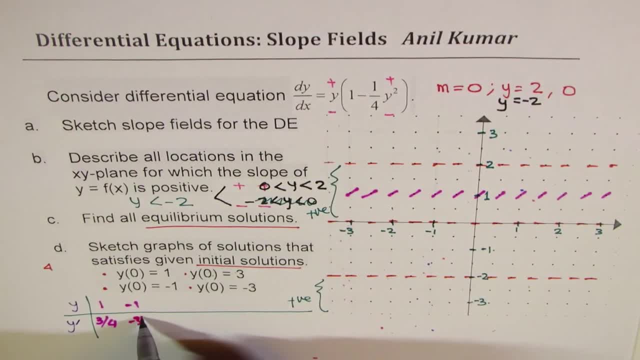 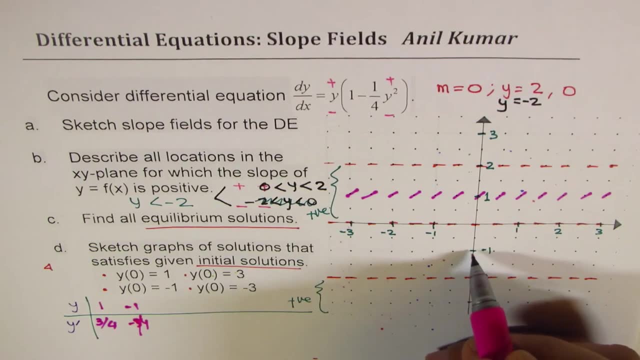 but that becomes negative three-fourth. right, So this becomes negative three-fourth. Do you see that Negative three-fourths? So instead of rising up at minus 1, it will be going downwards, correct? So it is kind of like this: Slightly less than 1, but downwards. So that is what it is. 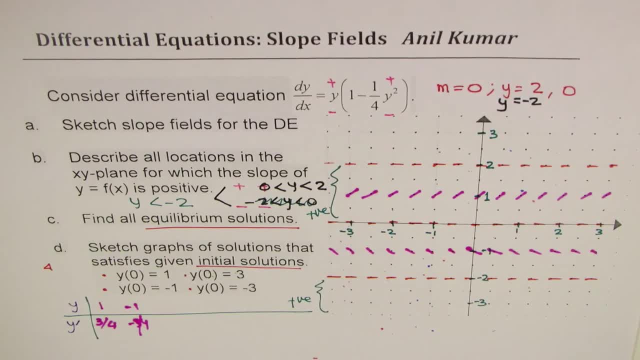 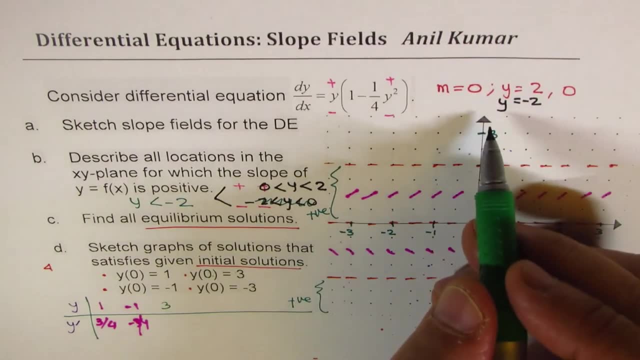 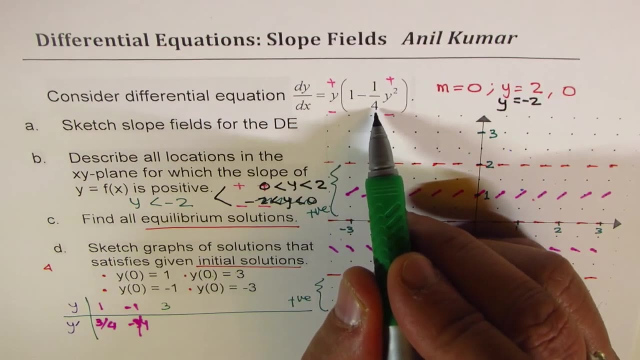 So you see a kind of symmetry here, right? Okay, Now let us take the slope when y is 3.. So if y is 3, in that case positive 3, this is positive. But here 9 over 4 will make this as minus 5 over 4,, right So? 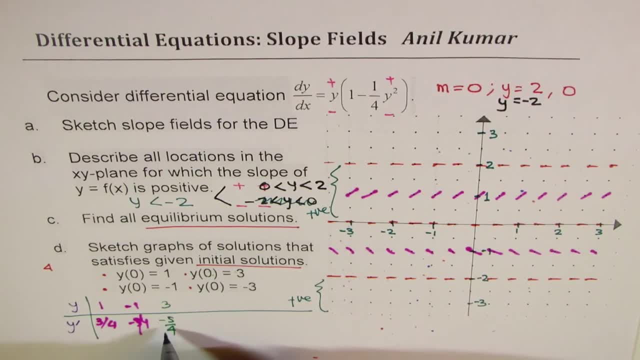 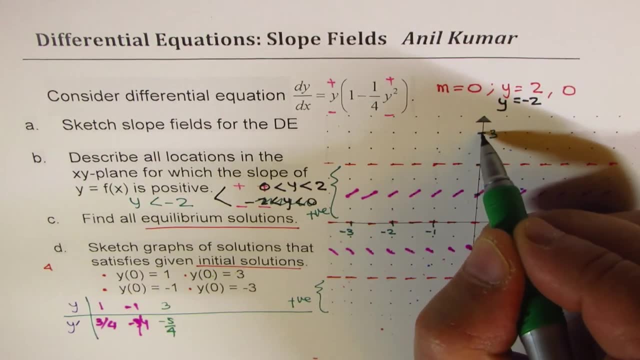 it is minus 5 over 4.. So slope is negative and slope is more than 1, right, So it is coming down negative and it is more than 1.. So let us say it is kind of like this: 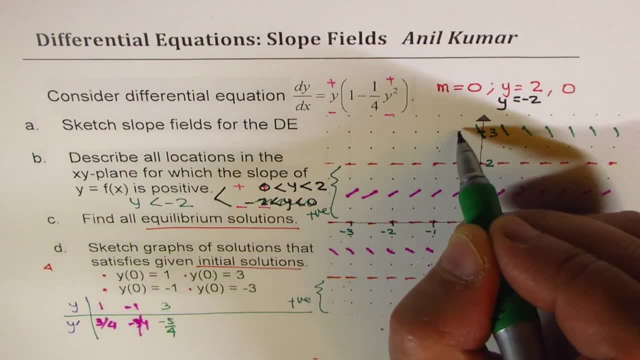 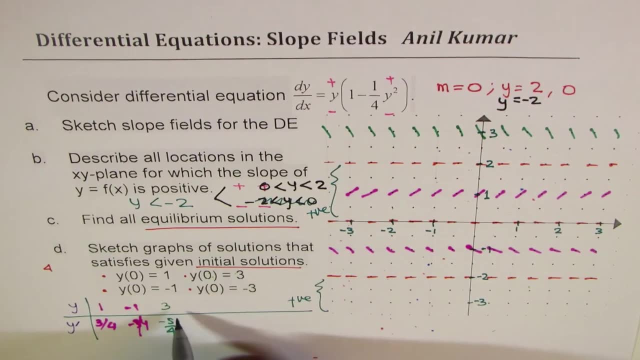 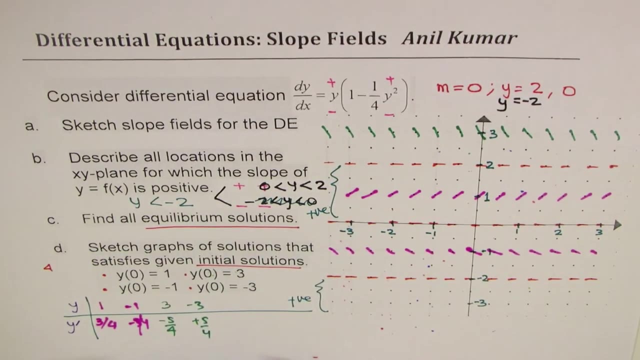 Since it is independent of x all along. y equals to 3, we can draw these short segments indicating the slope fields. Now let us look into minus 3.. For minus 3, it will only become plus 5 by 4,, since that becomes negative, right, So negative, negative. 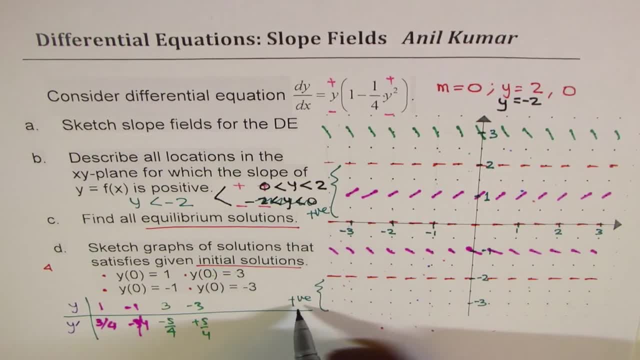 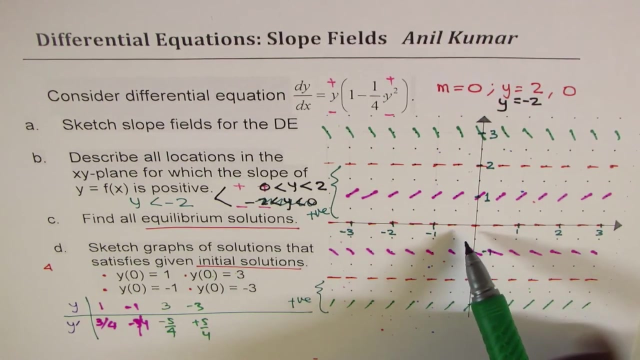 makes it positive. So for this now we are expecting positive, as we thought of. So we have positive greater than 1.. Correct, So we have more or less filled in the slopes. Now we could take values, 0.5 values also. 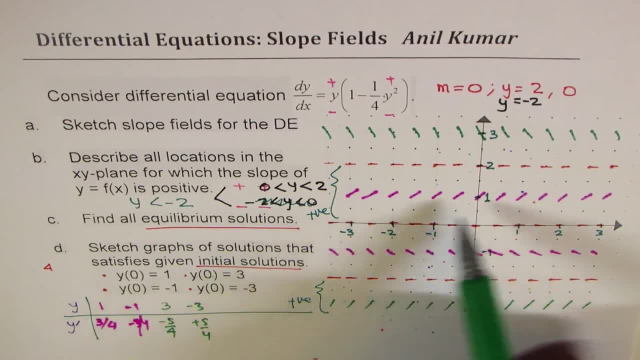 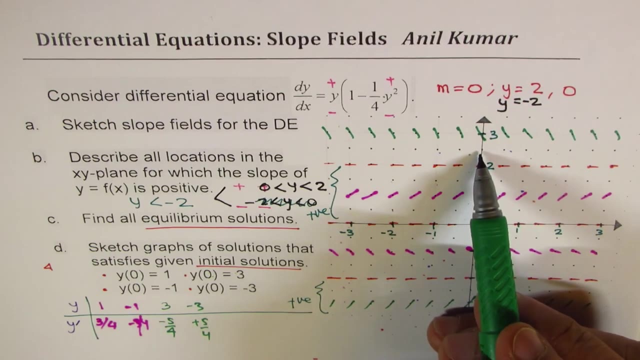 in between to fill up these gaps right And then get a better graph correct. Now the idea is that as the y value is becoming between greater than 2, we are having negative fields correct? So if I have 2.5, in that case we are getting negative fields. So if I have 2.5,, in that case. 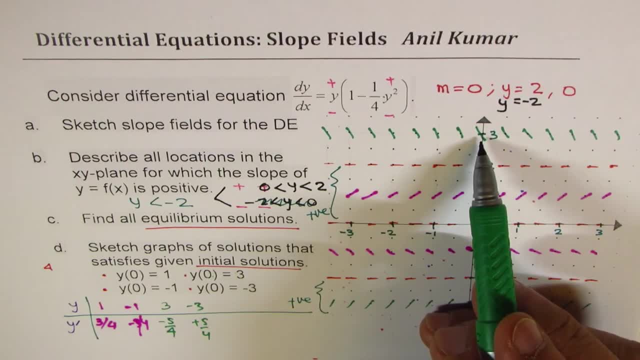 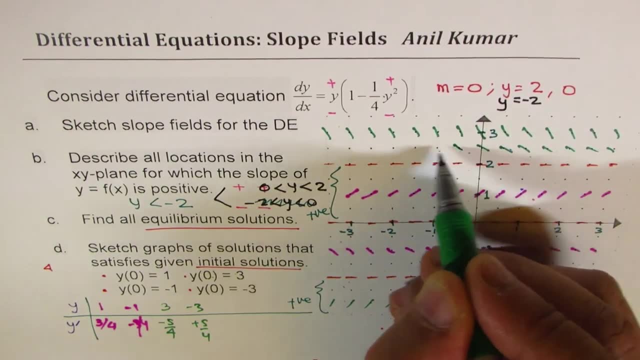 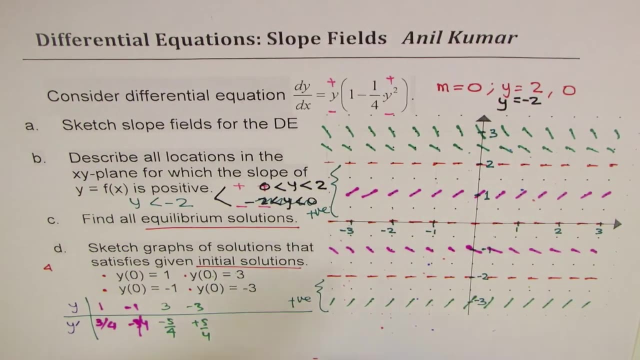 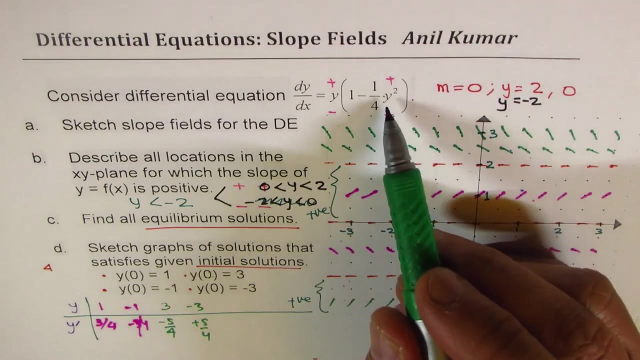 the slope will be slightly lesser than this, So we could do it like this: lesser than this, and we can just mark it here, right? So that is how the slope will be And similarly, here, if it is, the y value is less than 1, it is going to be more because that is. 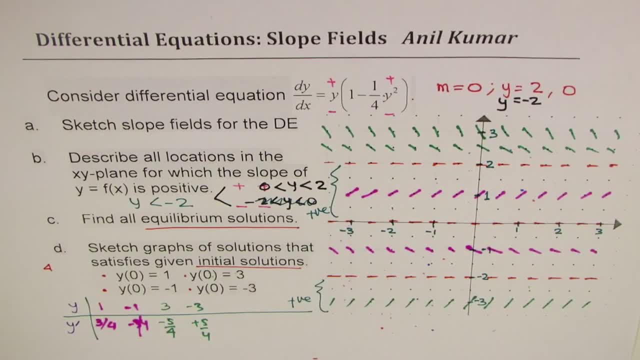 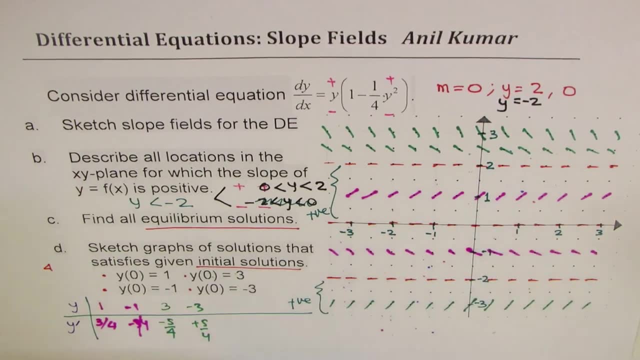 the minus 1 value. You can calculate all these values and figure it out correct Now. so that is how we kind of get our field. Now the question here is sketch graphs of solution that satisfies, given initial condition y 0, 1.. Now it means what? 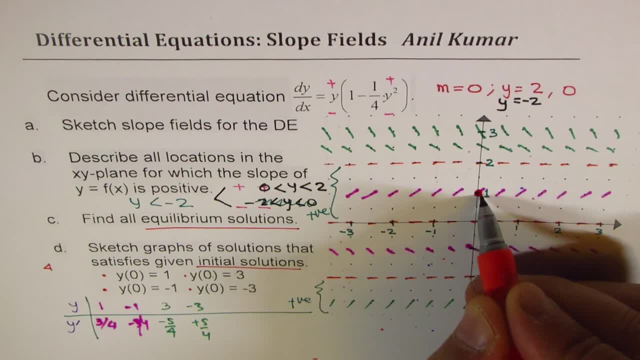 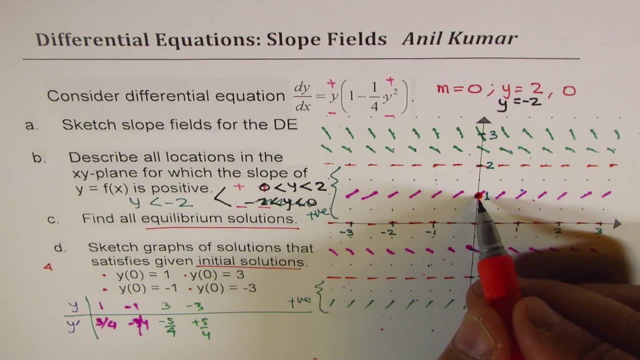 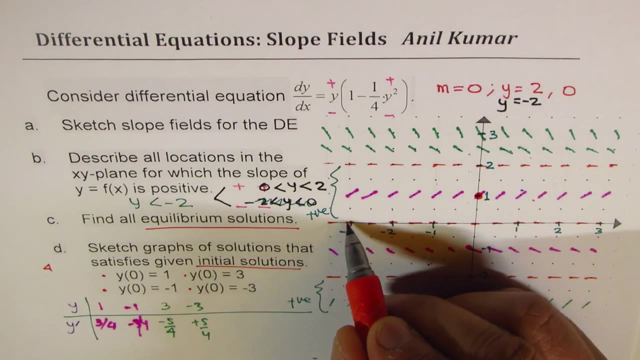 x value of 0,, y value of 1.. That means you are here. So this point is on your solution. How will the solution look like? That is what it means. So if you have to draw a slope field from here, then you know it is going to be tangent to this. 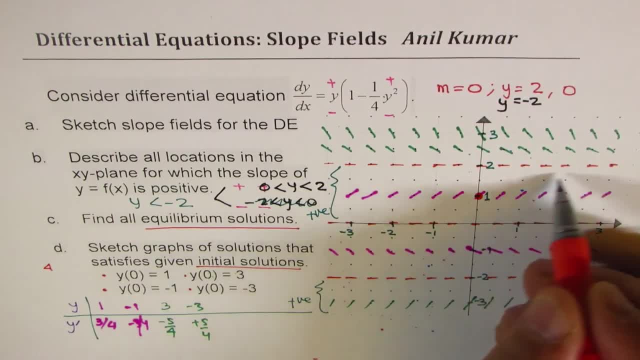 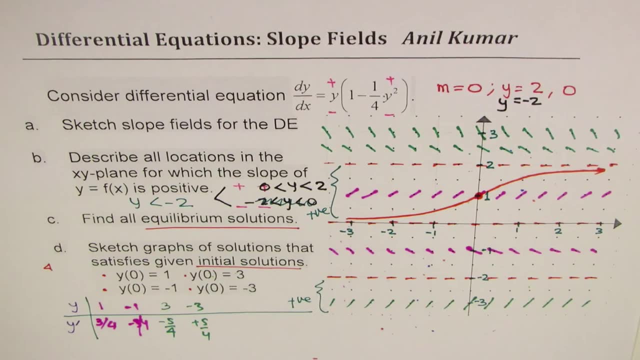 It is rising as you go up and then like this: That is how it is. So the slope will be kind of like this: Do you see that? So for this, that is going to be the particular solution when the initial condition y 0 equals to 1 is given. 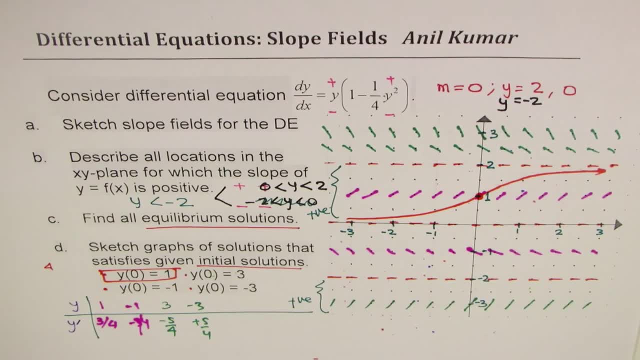 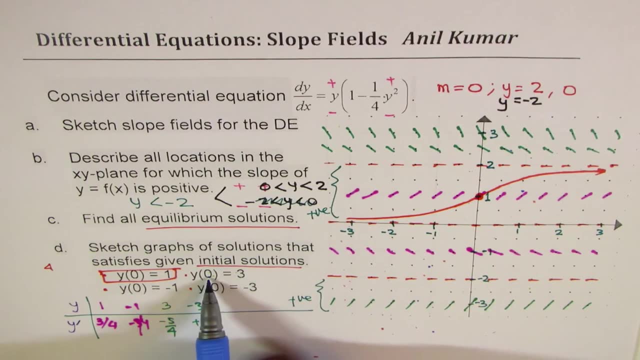 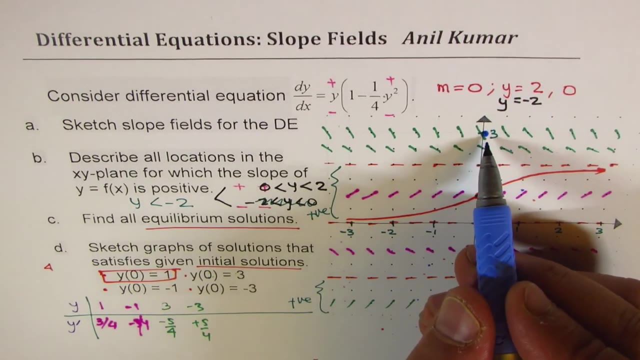 Got it. Now let us draw another curve. when y is 0 and x, y, 0 is 3. That means that x equals to 0, y value is 3.. So when we are talking about this point now, So at this point we know the slope. 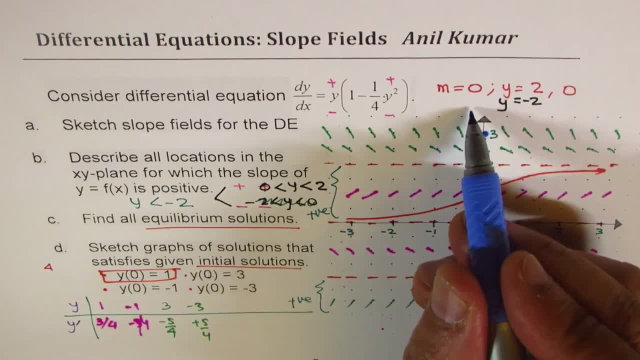 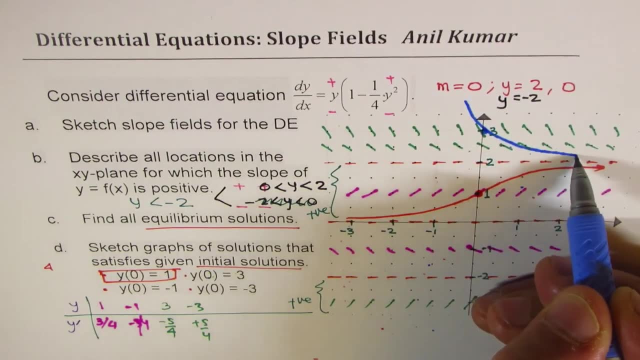 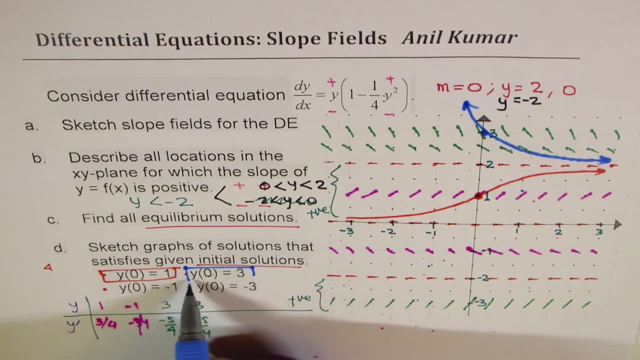 is negative, that the graph is coming downwards, right. So when we draw it it is going to be: these short segments are going to be tangent, So it has to be kind of like this: So that becomes the graph of the function going through 0 and 3, correct. Now let us take 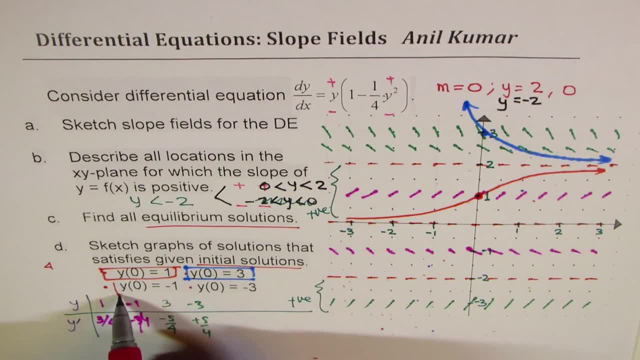 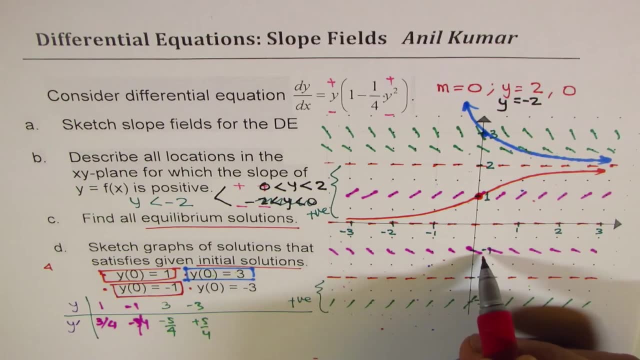 another ink and draw the next one, which is for 0 and minus 1.. So at 0 and minus 1, we are looking for this type of a function right Now. here you can see we are approaching this point. The. 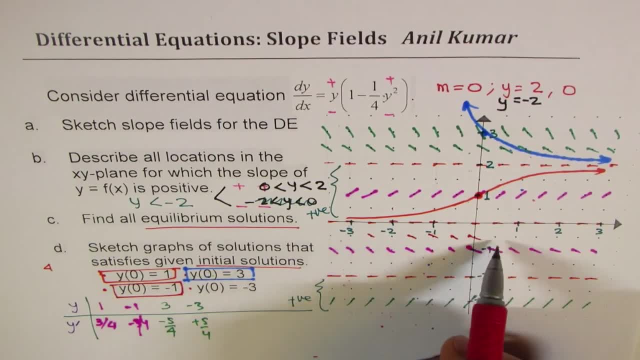 field here which I should have drawn will be kind of like this: You can calculate these values right, So it will be kind of like this. So what will happen here is that when you go through the point which is 0 minus 1,, 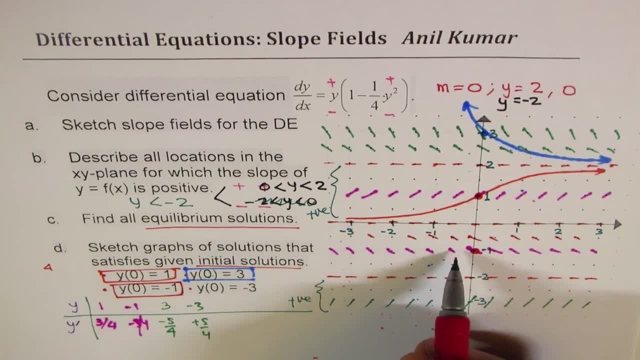 0 minus 1 is right there. In that case, the graph is going to be like this, So it will be like this. So you have to fill up these values to really get to see how it should be looking like. 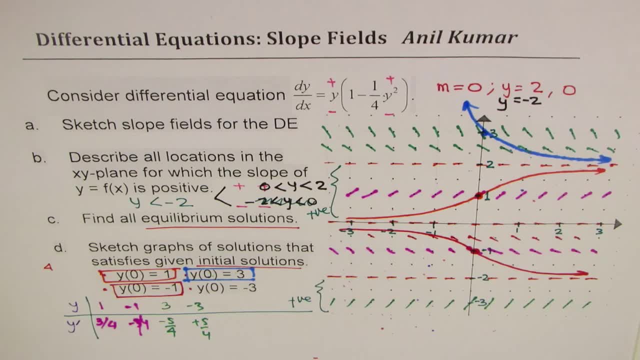 Is it okay, So you should do that part on your, on your own. The last graph here is when y value is 0 and minus 3. That means here all these functions are positive. It is a rising curve and it rises to equilibrium position of. 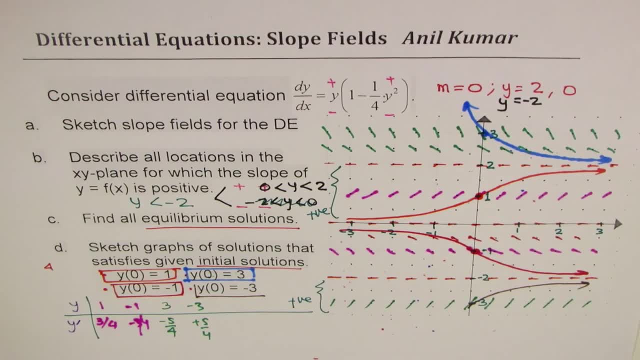 minus 2.. So it is kind of like this. So that is how you could get particular solutions when initial condition is given to you. So in this video, what we learn is that slope fields give us a look and feel of the slope. So in this video, what we learn is that slope fields give us a look 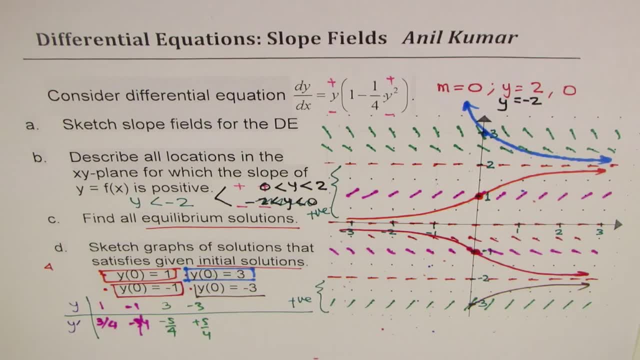 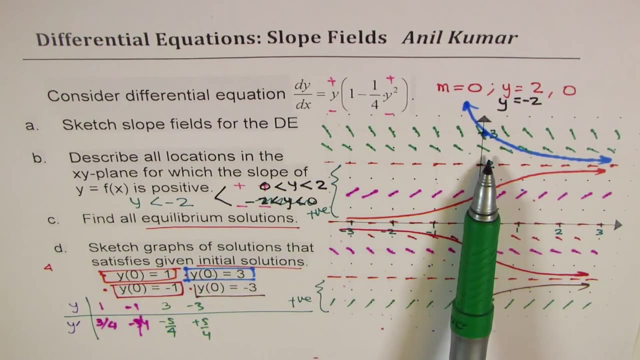 and feel of differential equations. They are easy to draw since the derivative is given by the coordinate function itself. So once you plug in the values of coordinate, you know the slope at that point makes short segments. at that point, Once you make all the short segments, you can.